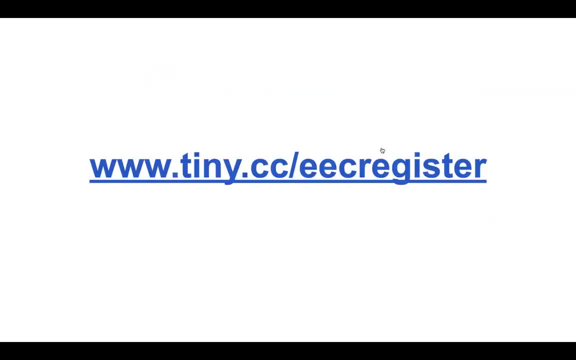 trip experience. If you are watching this and have not registered for this field trip yet, you can still do that. How you do that is by going to wwwtinycc slash eec register and once you get there, you can fill out a short form to get yourself or your class registered for this. 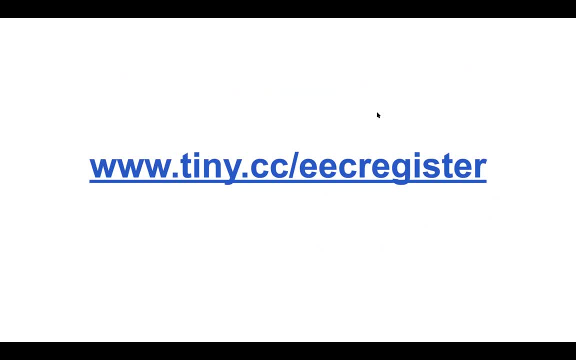 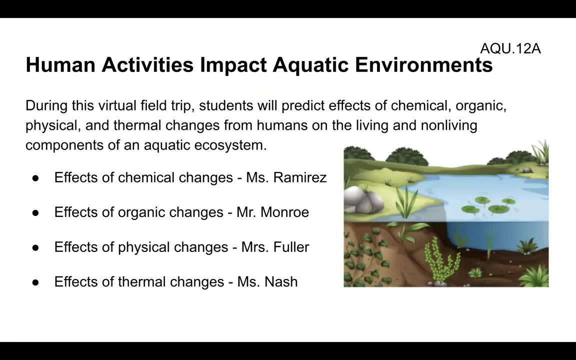 field trip. We just use that information for our attendance purposes. This virtual field trip is going to be about how human activities impact aquatic environments. During this virtual field trip, students will predict effects of chemical, organic, physical and thermal changes from humans. 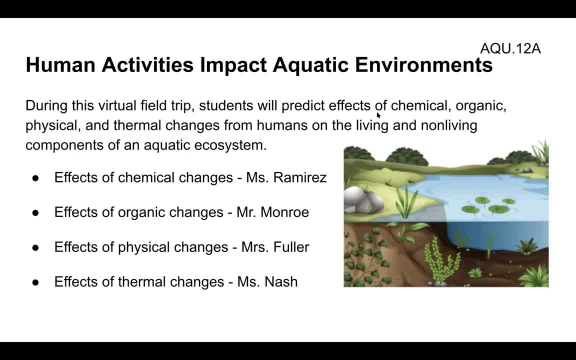 on the living and non-living components of an aquatic ecosystem. So first we're going to investigate the effects of chemical changes on an aquatic ecosystem, First we're going to investigate the effects of chemical changes on an aquatic ecosystem. That's going to be led by 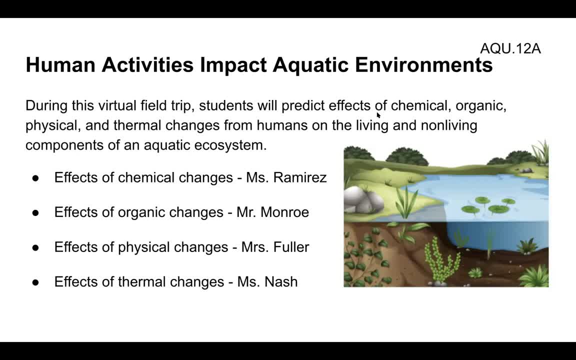 Mr Ramirez. Next we will investigate the effects of organic changes with Mr Monroe, Then we'll investigate the effects of physical changes with Mrs Fuller, And last we're going to investigate the effects of thermal changes on an aquatic ecosystem with Ms Nash. While we're 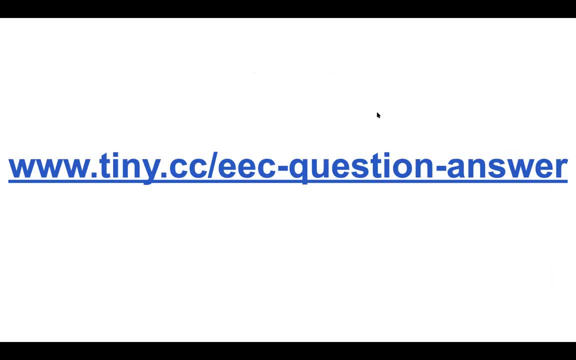 doing all of that. you can ask us questions. The way you do that is by going to wwwtinycc- slash eec, dash question, dash answer, and there you'll get to a very short form. Or you can type in any questions you have for us. You can ask us as many questions as you like and 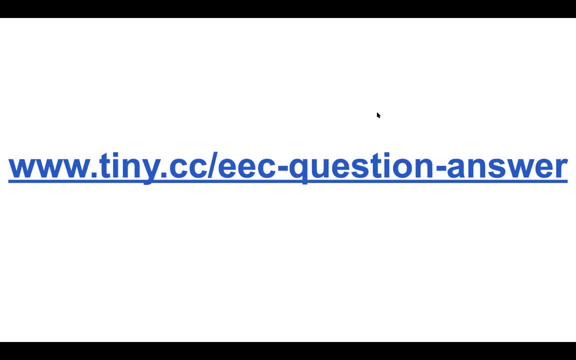 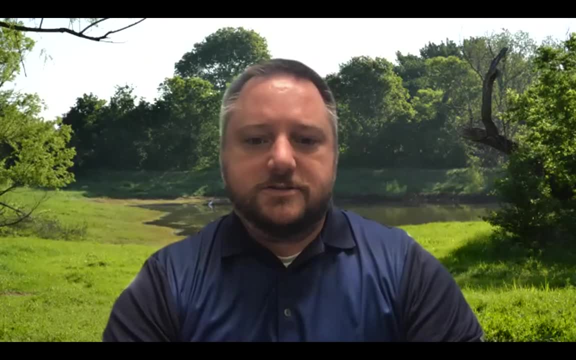 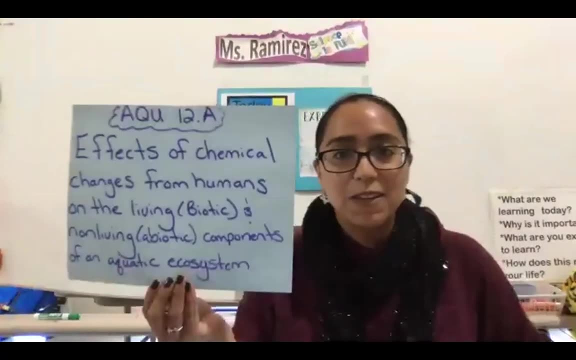 we'll do our best to answer all of them in the time that we have with you this morning, So let me stop sharing my screen here and we'll get started with the investigation with Ms Ramirez. Hello, my name is Ms Ramirez, and in this segment we're going to be learning about the effects 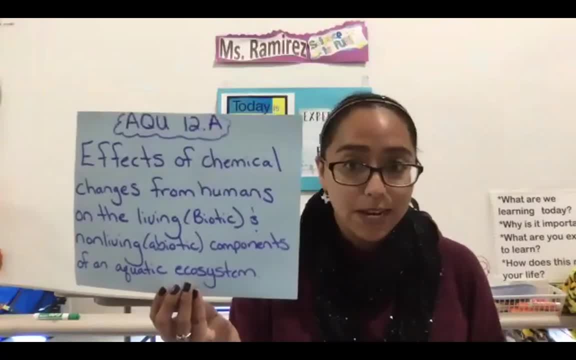 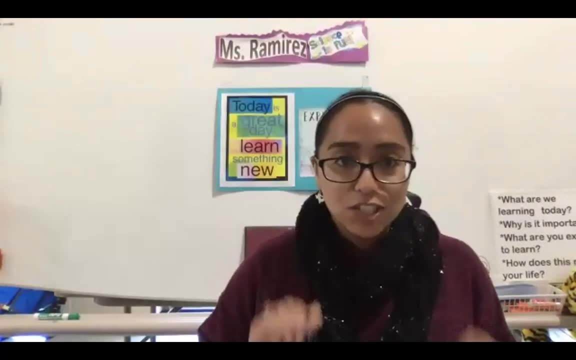 of chemical changes from humans on the living or biotic and non-living or abiotic components of an ecosystem. So what I'm going to do, I'm actually going to share my screen and we're going to look at a couple of pictures and some examples of chemical changes that occur here at the 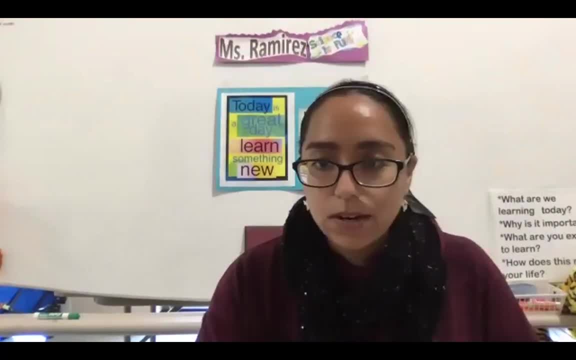 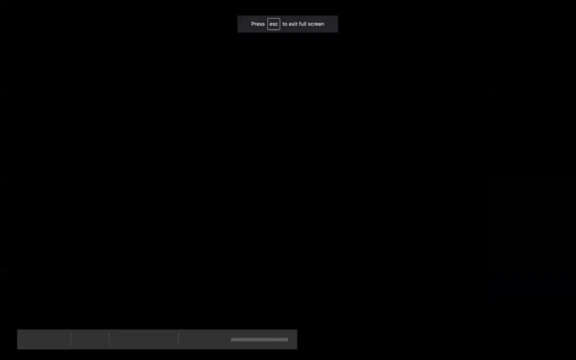 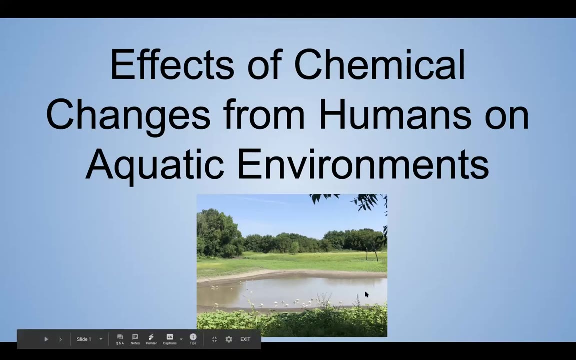 Environmental Center. So let me start our screen share, And here is our little PowerPoint, So let me go ahead and present that for you guys. So again, we're learning about the effects of chemical changes from humans on aquatic environments, And then, in this little picture here, we have an example of our pond that we used to have. 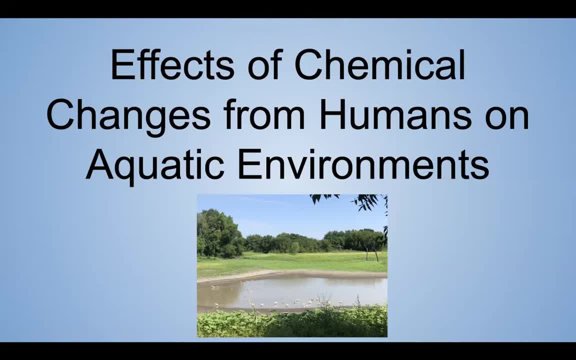 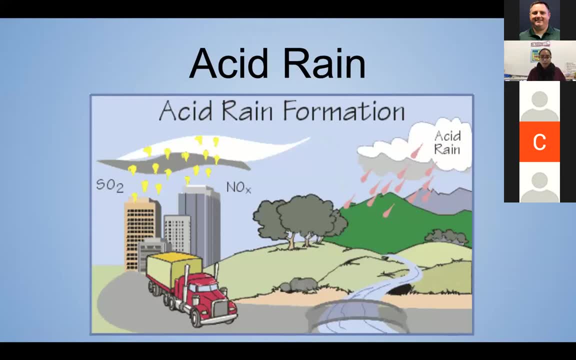 Unfortunately, it's no longer there due to drought, but, just like all aquatic environments, it is subject to changes from human impact. So the first thing that we're going to talk about today is acid rain, And acid rain results when sulfur dioxide- and in this slide it's represented by CO2, and nitrogen oxides are emitted into the. 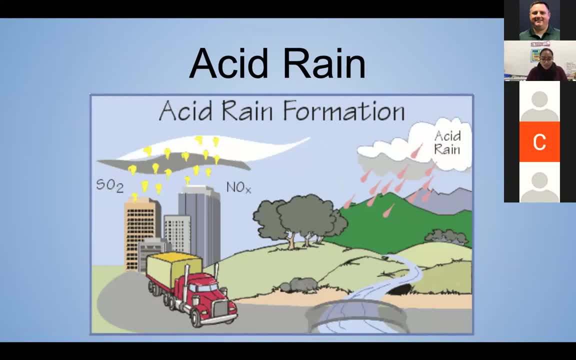 atmosphere and transported by wind and air currents. A small portion does come from natural sources such as volcanoes, but almost all of it comes from the burning of fossil fuels, And we use that burning of fossil fuels to generate electricity. It becomes emitted in our vehicles and also in manufacturing and oil. 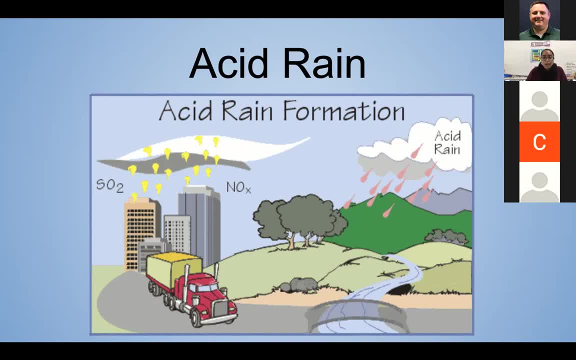 refineries are another source of sulfur dioxide and nitrogen oxides And it's important to note that when I say the word acid rain, I know that sometimes there's a confusion with students. So it's important to note that when I say acid rain, I'm not talking about like super dangerous. 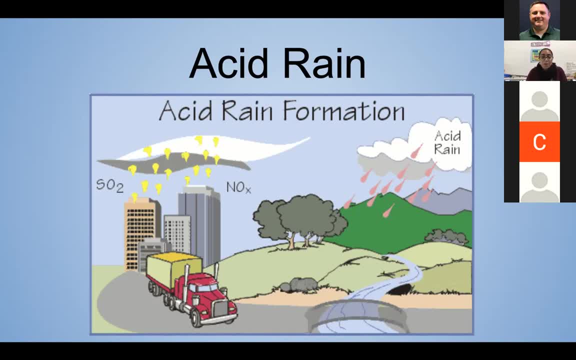 acid that's going to burn or hurt you. Um, you can actually walk out in acid rain and in- and- and typically our own rain is actually on the slightly acidic side, So it's not super dangerous, but over prolonged periods of 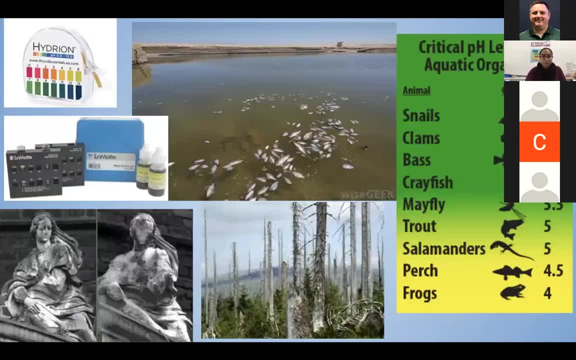 time it is very harmful to the actual environment. So let's look at some effects of acid rain and how it harms the environment. So here we have some examples of some fish that have died due to differences in acid levels. So we take a look at our PhD level. 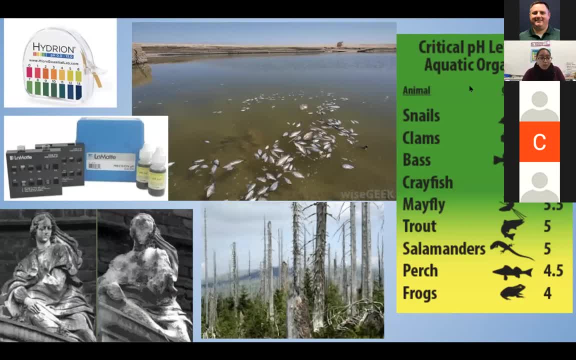 levels for aquatic organisms. certain organisms can only tolerate certain pH levels. So if you've ever looked at a pH chart, you'll notice that seven is neutral and then anything between one and six is considered acidic and anything between eight and 14 is considered basic. So if we look at 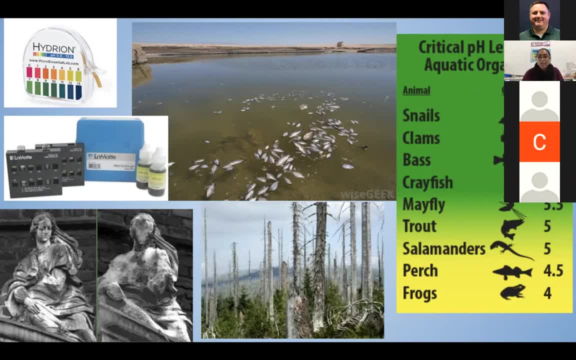 our chart over here for aquatic organisms, you can see that snails and clams prefer a pH level of around six. Bass, which we have a lot of, or we used to have a lot of, in our ponds over here, prefer about a pH of five and a half. So five and a half is actually just slightly acidic. 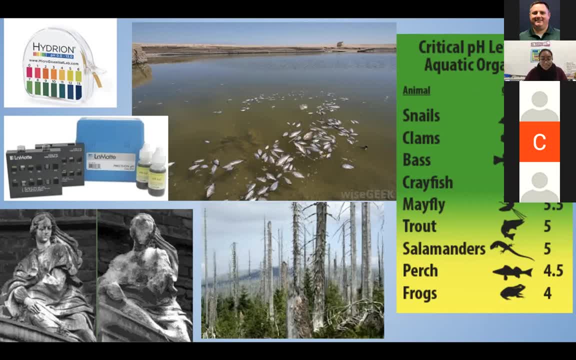 and again. our typical rain is just slightly acidic. Now acid rain itself is going to have a pH of around four. So if we have high amounts of acid rain and the pH is four, these other organisms are not going to be able to survive for prolonged periods of time under those unfavorable pHs. So if we have a pH of four, then we're not going to be able to survive for prolonged periods of time under those unfavorable pHs. So if we have high amounts of acid rain and the pH is four, then we're not going to be able to survive for prolonged periods of time under those unfavorable 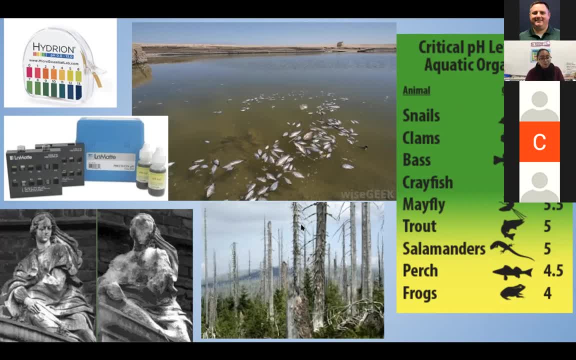 pH conditions. Now, pH can also affect the trees. So when we have acidic rain, that rainwater will leach into the soils and it will affect how our trees grow. Now the acid rain also affects statues and buildings. So you can see here it's starting to dissolve or eat away at some of the 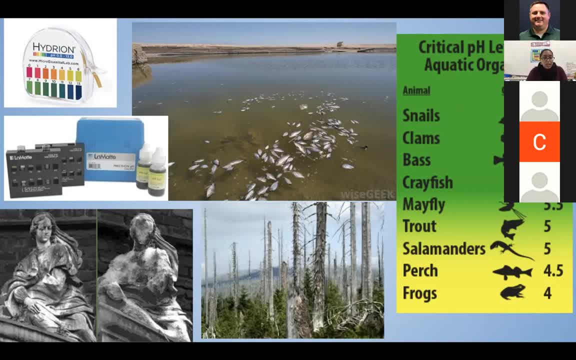 limestone and other rock formations. And then, if you joined us in our previous webinar, you saw how we measured the acidity or the pH level of aquatic systems using pH. So if we have a pH of four, then we're not going to be able to survive for prolonged periods. of time under those unfavorable pH conditions. Now pH can also affect the trees. So when we have high amounts of acid rain and the pH of four, then we're not going to be able to survive for prolonged periods of time under those unfavorable pH conditions. Now pH can also affect how our trees grow. 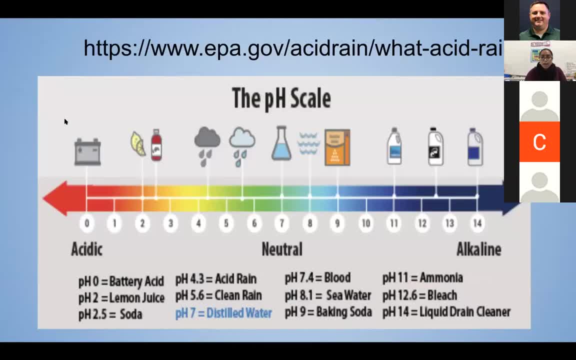 And those are an example that you see here. Now, in our next slide, that's the actual pH scale And this is just to show you an example of the different pH levels of some common household things. So remember, seven is neutral, Typical rain by itself, clean rain. it's going to be around. 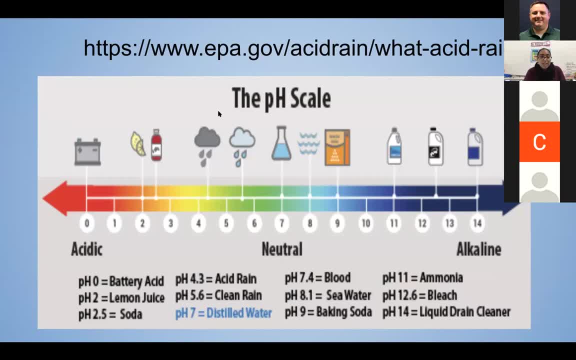 five and a half or 5.6 for its pH, Acid rain is going to be more along the lines of four to 4.3. And if you compare that to things like lemon juice, lemon juice or lemon juice, it's going to be. 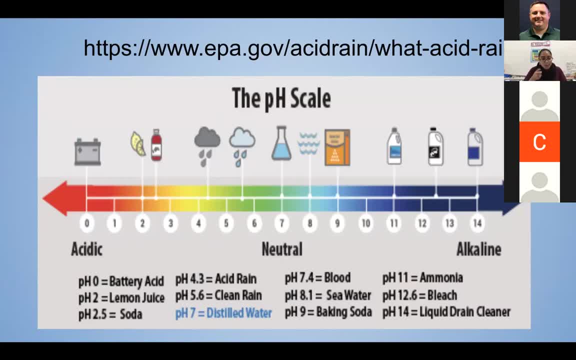 more like two. So you're going to see that the lemons themselves have a pH of two. So that's why sometimes when you're squeezing a lemon, if it gets inside your eye it might burn or sting a little bit, So that is acidic. And then on the far end of the pH scale for things that are highly 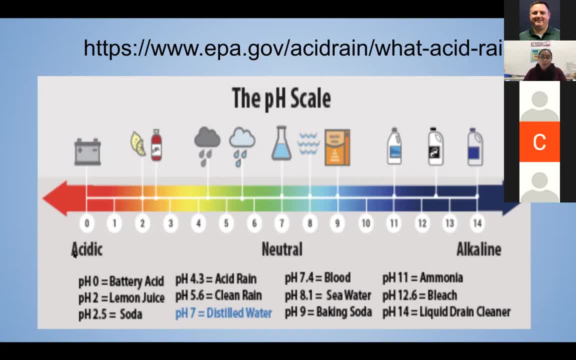 acidic would be things like battery acid, And those are super corrosive and also very dangerous to come in contact with. And then, on the other end, we have things that are alkaline or basic, So that would be things like bleach, ammonia, baking soda which we used in an experiment. 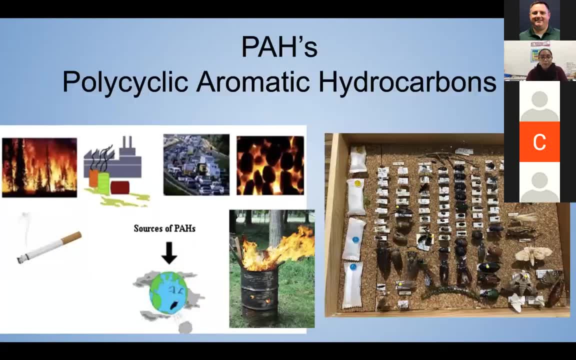 earlier today. And then on the other end, we have a lot of things that are alkaline or basic day, So that's the pH scale. And then another type of chemical that affects our waterways is polycyclic aromatic hydrocarbons. I know that's a big word to say, but these are chemicals that 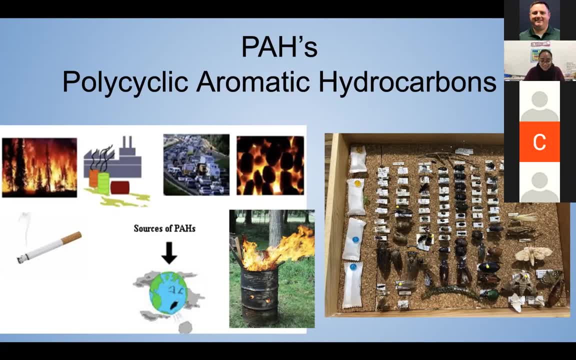 occur naturally in coal, crude oil and gasoline. It's also produced when coal, oil and gas, wood and garbage are burned. And then I'm born and raised in the city, so when I moved out to a rural area I was surprised to see how many people burned their garbage. So what I learned? 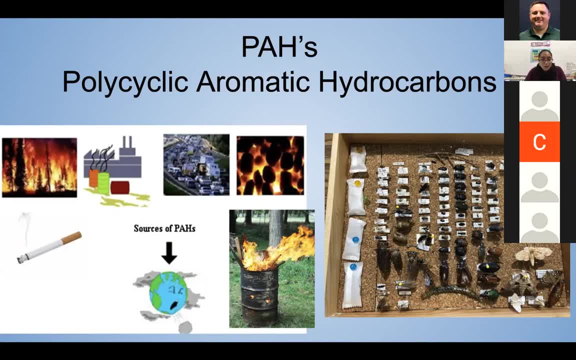 based on the EPA website is that burning of garbage actually releases a lot of these PAHs into the environment. So it's not really a good idea to burn things like plastics, because it releases a lot of those hydrocarbons into the environment. And something that I didn't 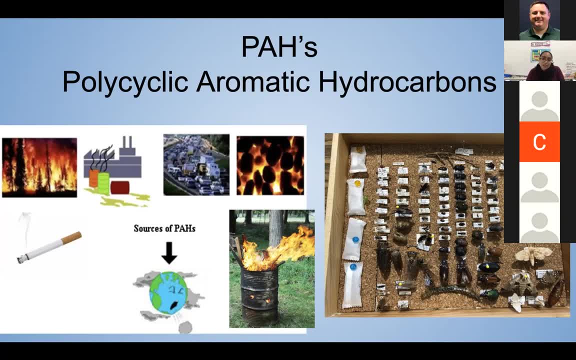 realize until now was that a lot of these polycyclic aromatic hydrocarbons I used to make dyes, plastics and pesticides, And one of the common things that I actually am guilty of using a lot of are these moth balls, And I use these moth balls during the summertime. 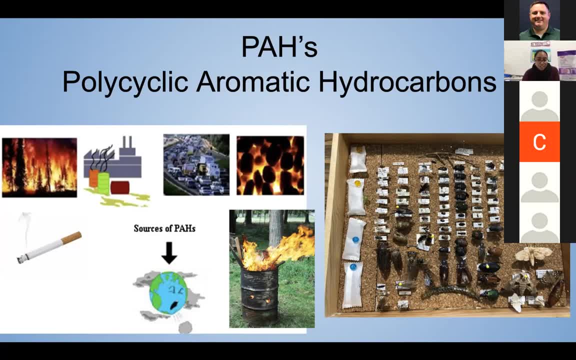 because we use them for our insect collections that we use during our summer program. So here's an example of one of my insect collections and all the moth balls that I've used in there. So again, I didn't realize that a lot of the products that we use actually have those PAHs. 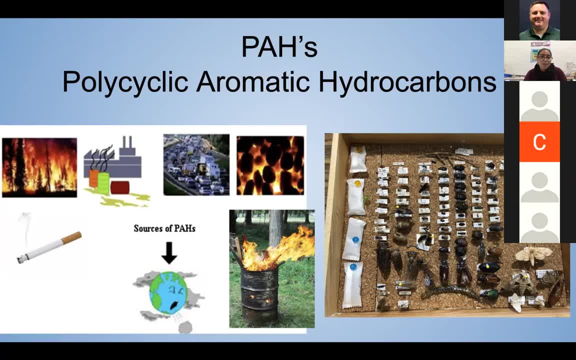 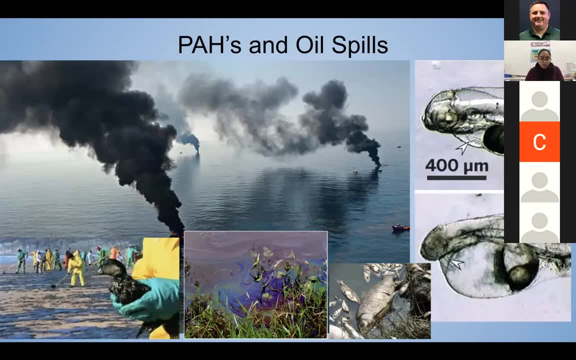 in them, And then another common source of polycyclic aromatic hydrocarbons would be things like the oil spills. So we all remember or hear about that big oil spill back in 1989, the Exxon Valdez oil spill, And then also that 2010 Deep 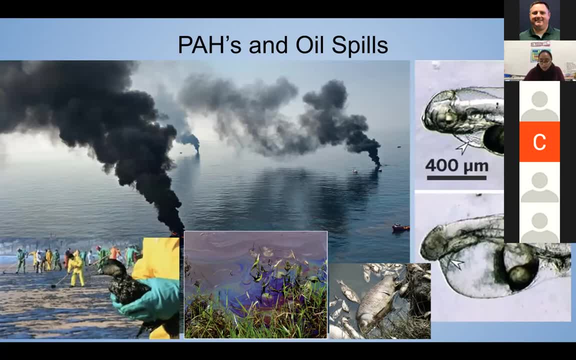 Water Horizon oil well blowout that left 168 million gallons of oil into the water, And so here you can see a couple of pictures that demonstrate the effects of oil spills on the environment. So you can see how, at a plant, both animals and plant life. And then these are actually some embryos of salmon, And a study was 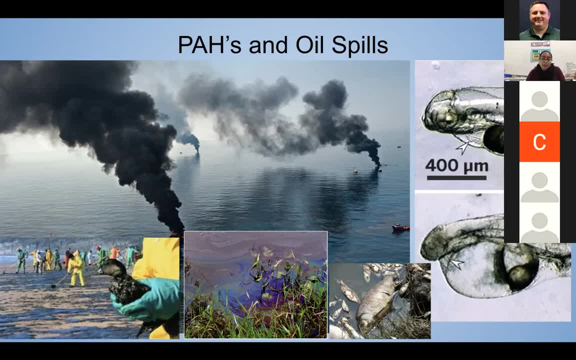 conducted to see how oil spills affected salmon And it showed that their hearts were actually deformed and they had a lot of fluid buildup around their hearts and it was causing them to not live as long And it was also affecting their ability to swim as fast. So there's a lot of cool. 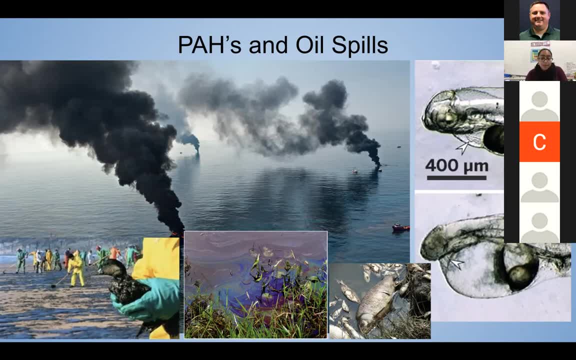 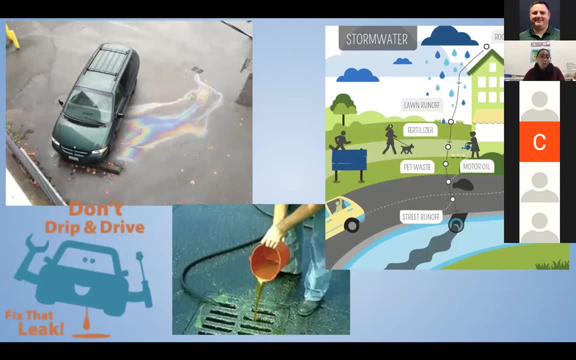 and interesting studies on how oil spills affect salmon, And I'm going to show you a couple of pictures that show how oil has affected plant and animal life. And then you might think: well, how do those oil spills affect me? Well, the cars that we drive have oil in them, And I'm guilty of. 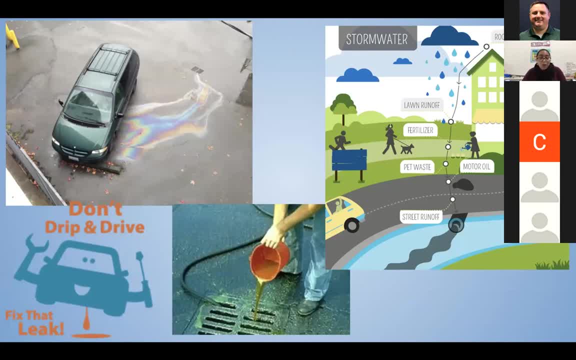 this too, because I actually had an oil hole in my oil pan and I was leaking oil last year. But you can see, if you don't regularly maintain your vehicle, the oil spill will actually travel and find its way to nearby water sources. So you can see that there's a lot of fluid buildup around the oil spill. 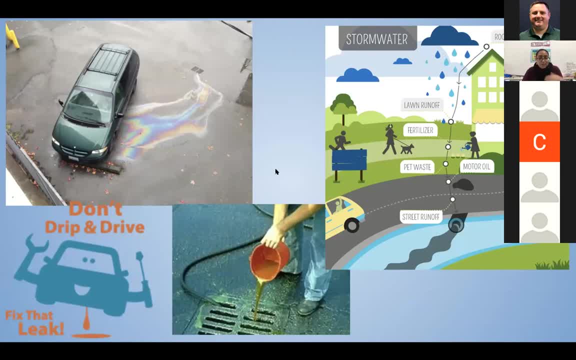 So you can see that there's a lot of fluid buildup around the oil spill And I'm going to show you a couple of pictures that show how oil spills affect salmon. And I'm going to show you a couple of pictures that show how oil spills affect salmon So you can see, if you don't regularly maintain your vehicle, the oil 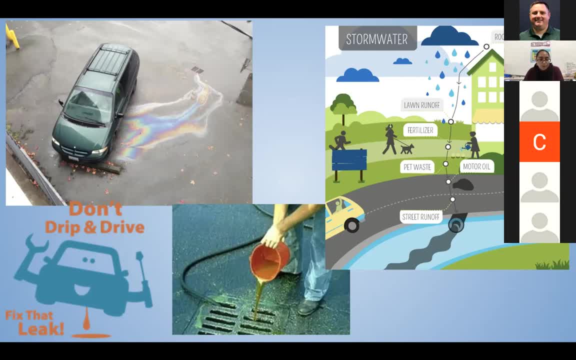 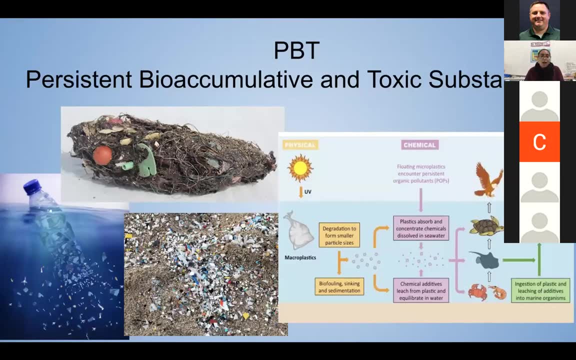 spill will actually travel and find its way to nearby water sources. And then also, if you clean out or change your own oil, to make sure that you're disposing of that oil properly and you're not just dumping into the drainage pipes or waterways. So that's also something to take into consideration. 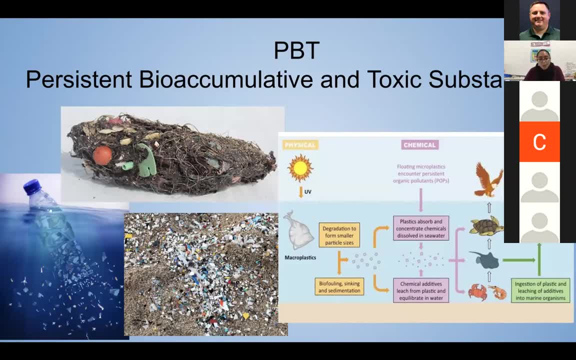 That's something that y'all can help do on a small scale. And then another chemical that plays a role: microplastics. So I know a lot of times you're walking through the neighborhood or you might see a pond or a lake and you see all those plastics floating around. Eventually, those things will 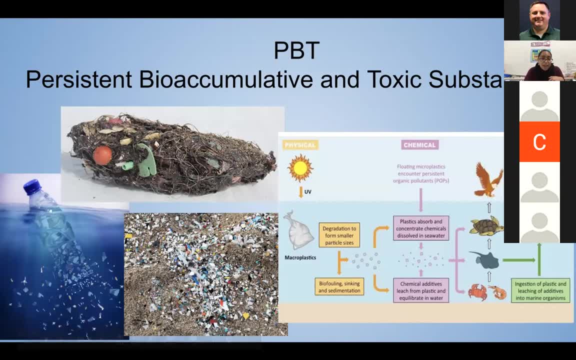 start to weather down or break down and we have what are called microplastics, And they're extremely hard to get rid of and it's very detrimental to the animals because they actually end up ingesting them. So what you see here is an example of an albatross bolus, And an albatross is just an. 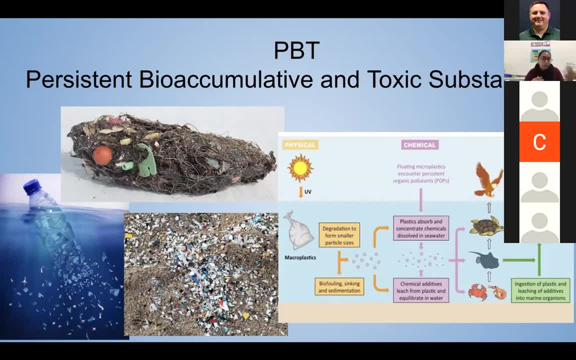 aquatic bird And a bolus. if you remember back to elementary school when you might have dissected an owl pellet, a bolus is something very similar. So whatever the albatross doesn't, whatever the albatross eats and its body can't digest, it will spit it back up in the form of a 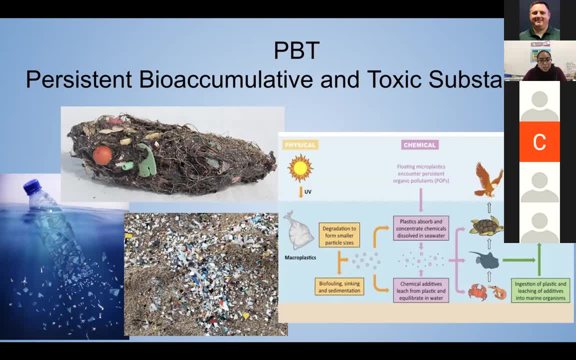 bolus And that is what you're seeing here, And scientists actually study those boluses because it tells us what they're eating. So you can see inside this bolus there's a lot of trash and plastic debris, So you can see how that. 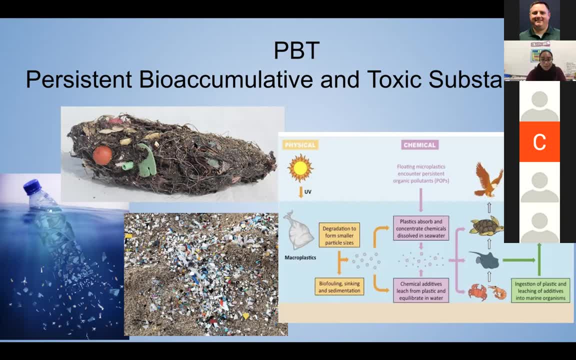 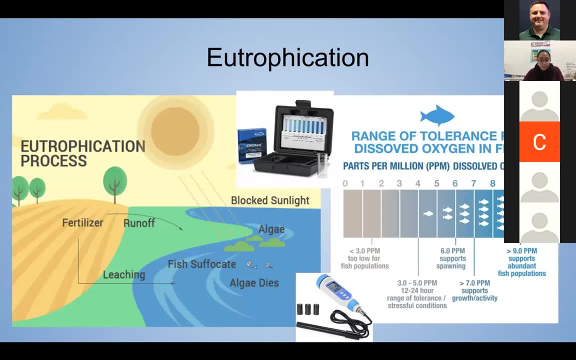 our trash impacts wildlife because they're ingesting it. And then the last thing, and this one pertains mostly to us here at the Environmental Center, and that's eutrophication. And eutrophication is simply when water becomes overly. 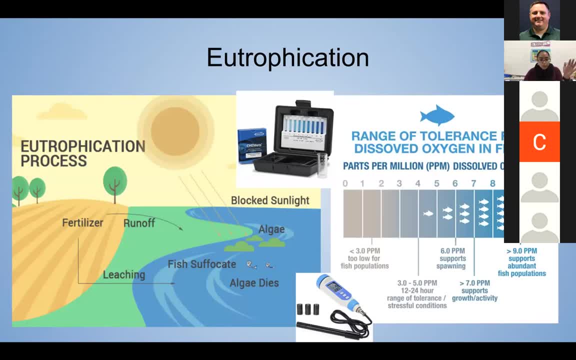 enriched with nutrients due to fertilizers. So when fertilizers from nearby farms, when that runs off into the waterways, it will eventually end up in our ponds and lakes and that causes an increased growth in algae. When we have too much algae, all that algae will block out the sunlight and it 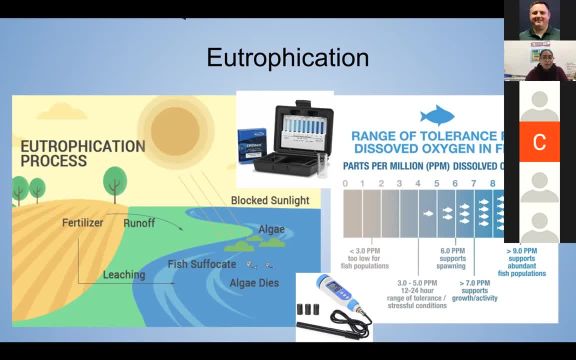 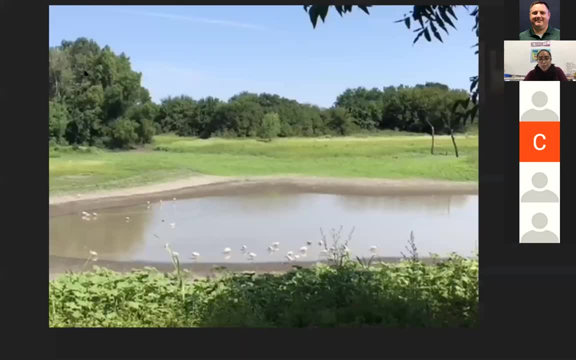 prevents other aquatic plants from growing. So what I'm going to go ahead and show you next are just a couple of pictures from out here at the Environmental Center, and we're going to relate that back to some chemical changes. So here's our pond that we used to have Again, it's now sadly dried up. 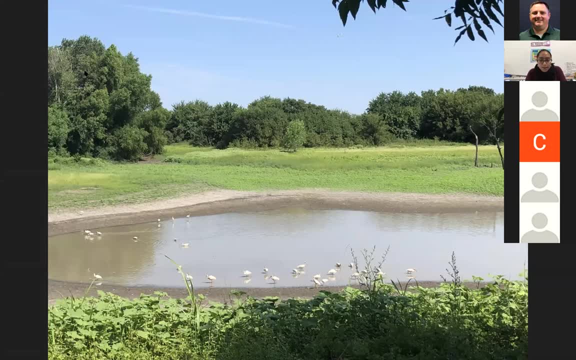 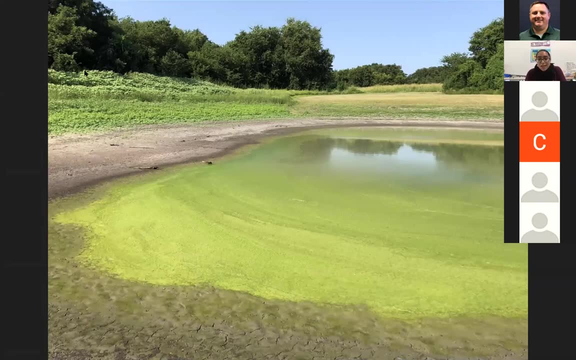 But that's our pond and those are some spoonbills that are feeding on some of the fish. Over time that pond turned into this, So you can see all that green algae and that was creating a very hypoxic environment, meaning there wasn't a lot of oxygen, so a lot of the 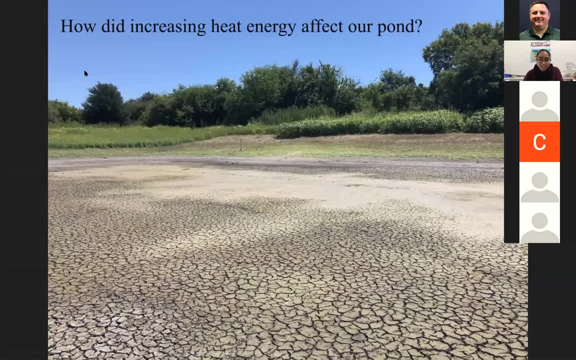 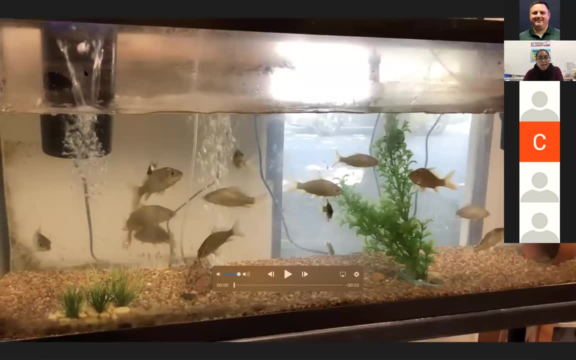 fish ended up dying off And that is what it looks like now. It's completely dried And again you can see the cracks. Those are some of the remains of the fish, skeletons, And a lot of people are surprised to know that fish and aquatic 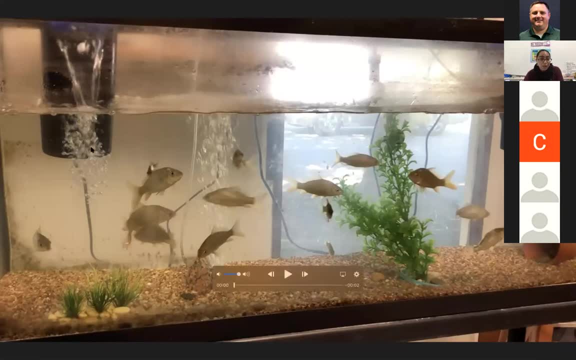 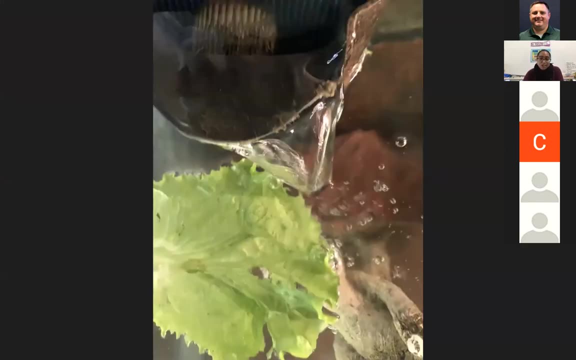 organisms need oxygen too. So if you've ever seen an aquarium, you see the filters with the bubbles. That's their way of aerating and adding oxygen into the water. So, yes, fish need oxygen as well, As well as our other aquatic organisms. And the last thing I want to leave you: 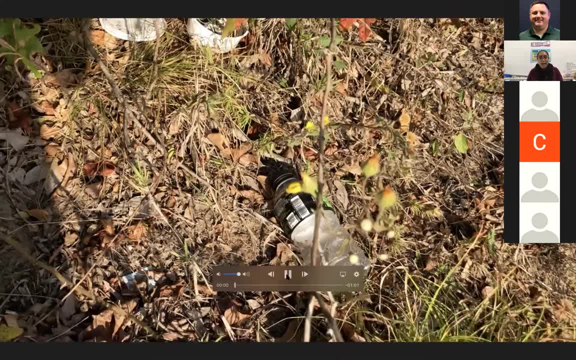 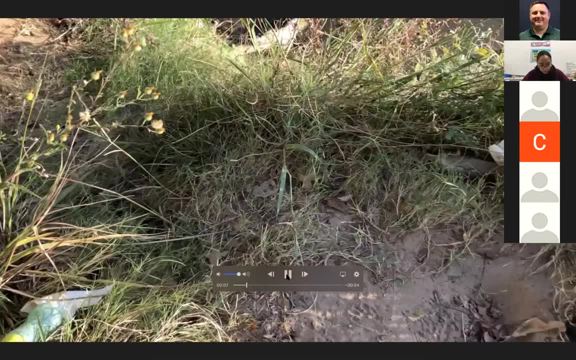 with is just a really quick video that I took over here at the Post Oak Preserve. It's a county park that's across the street from us, but you can see all that litter and trash. So my reflection question for y'all is: what effect have? 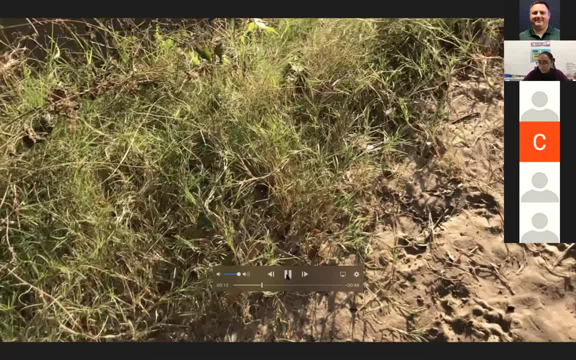 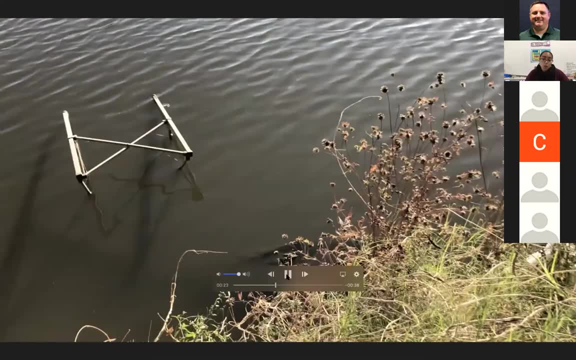 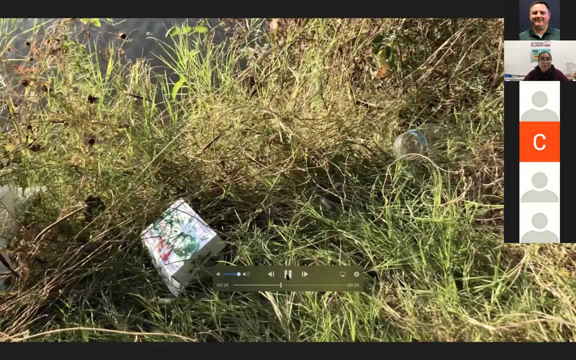 humans had on your local parks and green spaces And then also think about what can you do to help limit or remedy the negative effects that human might have on the environment. So it really is a beautiful preserve over there, but there is unfortunately a lot of trash. 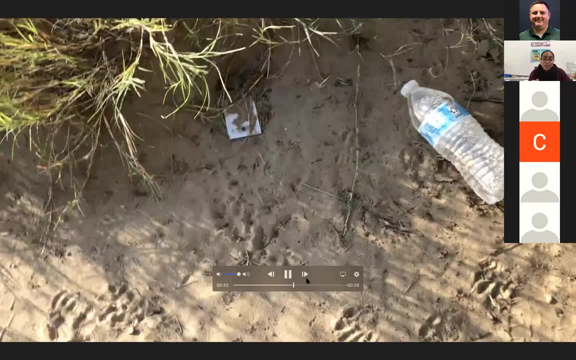 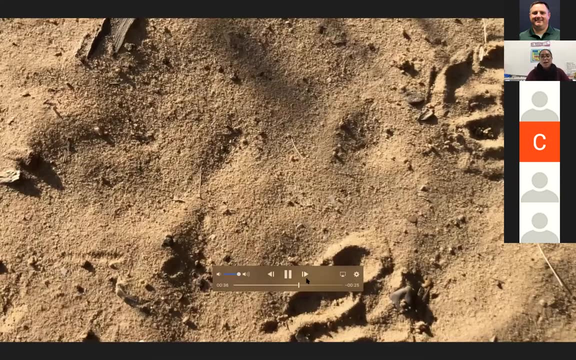 So be thinking about how does that trash affect our animals? And we can see an animal's been walking through there. I think those might be coyote footprints maybe. So we do have lots of wildlife in that preserve. I'm going to go ahead and stop it. 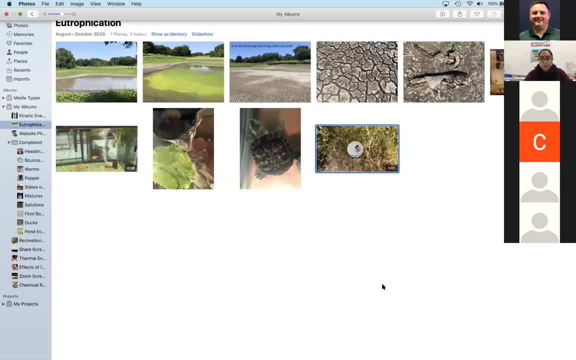 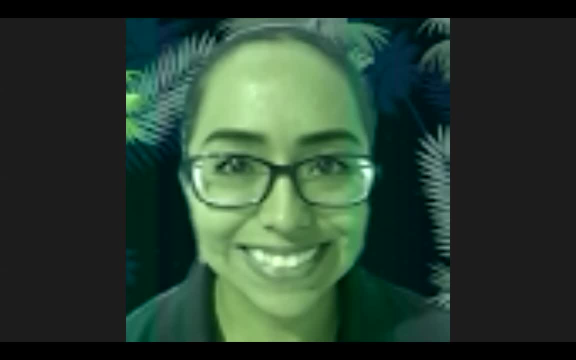 there and I'm going to stop sharing our screen And I'm going to go ahead and pass it back to Mr Broughton. He's going to answer any questions. Thank you, Mr Ramirez. The question that came up was: can microplastics get into the air And 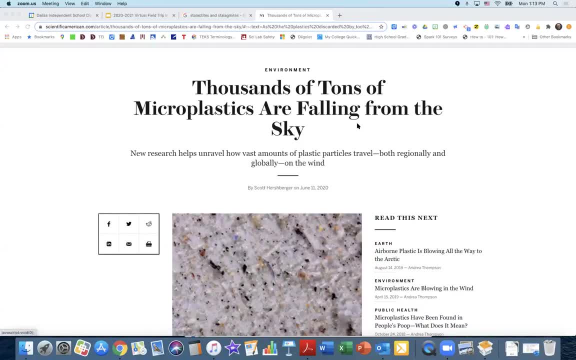 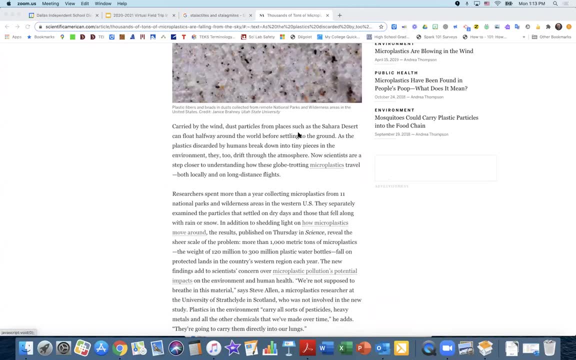 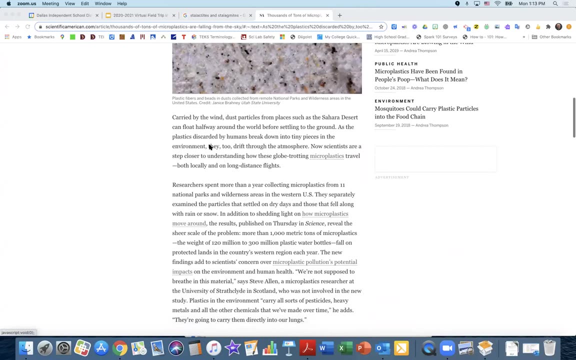 yes, they can. I'm going to share my screen with you real quick to show an article that explains that. So maybe you've heard of dust from the Sahara desert floating halfway around the world. I mean, that happens, and plastics too Can get blown up into the air. and moved around. So, like recently, some researchers spent a year collecting microplastics from 11 different national parks and they found a thousand metric tons of microplastics in those areas. So, yes, it can get in there. That's why it's so important not. 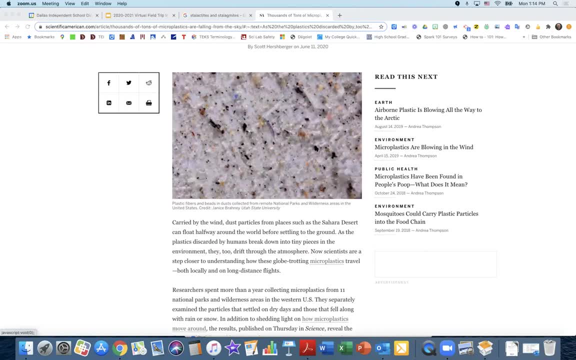 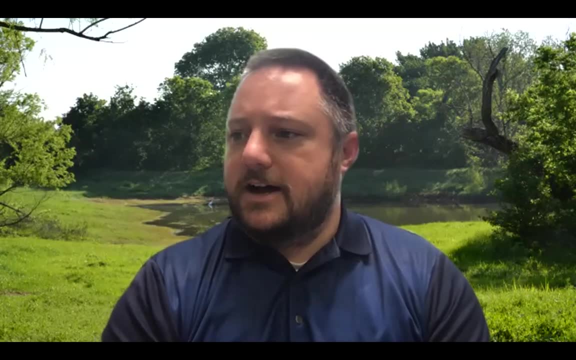 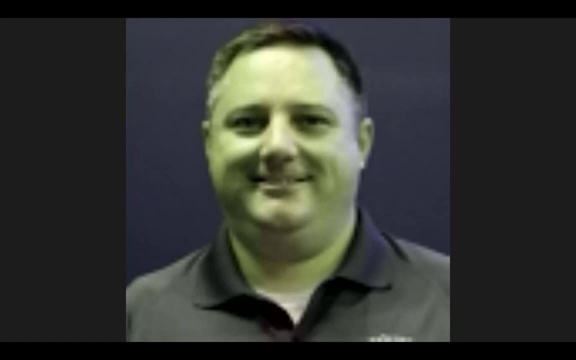 to litter and, if you do see litter, to clean it up. All right, now I'm going to stop sharing my screen here and we're going to move on to Mr Monroe, who is going to explain organic changes to aquatic environments. Good afternoon students. My name is Mr Monroe and 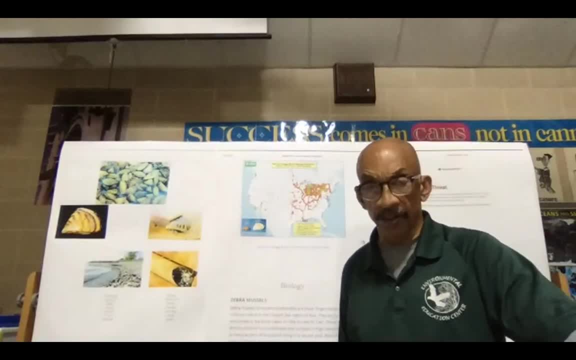 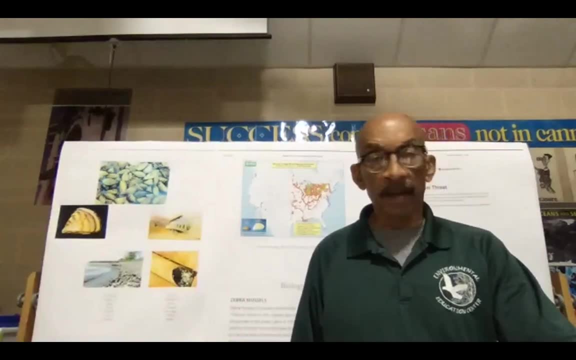 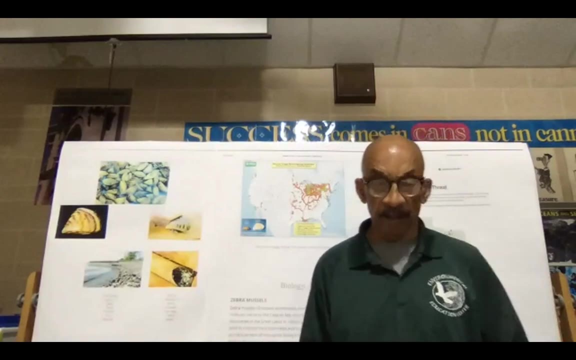 my portion of your virtual field trip today is to share with you and discuss with you about organic impact on our environment caused by humans. And you know there are certain indicators, just like the ponds that we had out here at the center, and we've got the 12-acre lake that's in the 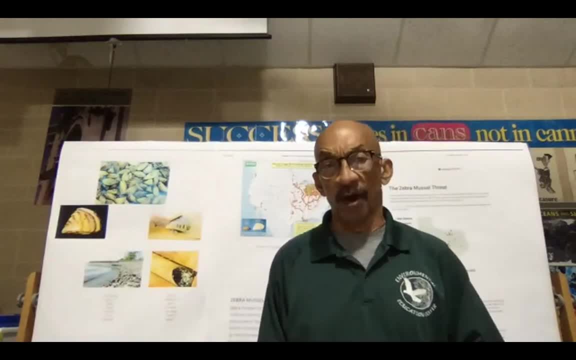 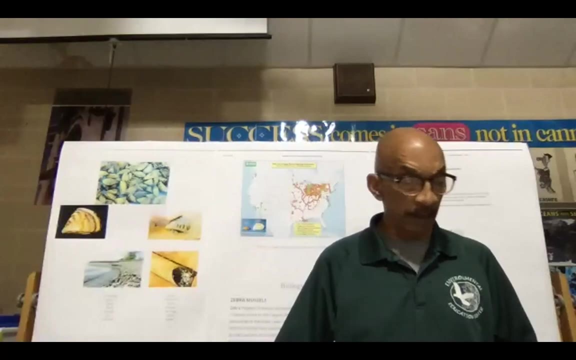 Postal Preserve, But there are other bodies of water there in this state that are infected or infested with a very invasive type of muscle, And they got infested simply because of the actions of human beings. Now we know that we use our lakes here in this state for a lot of things. 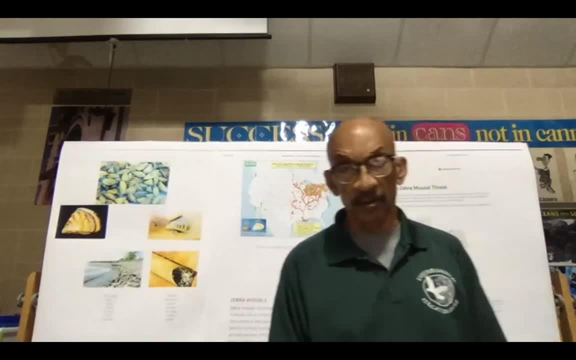 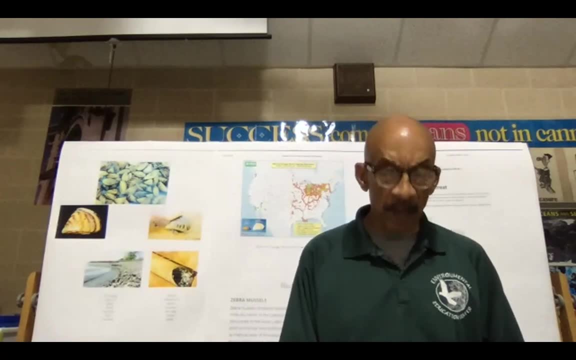 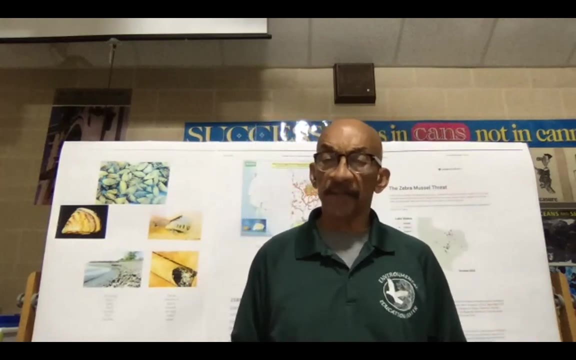 For a lot of different purposes- Recreation, industrial, municipal- and we have a tremendous impact if we don't take care of it. Well, usually with water quality, believe it or not, there are certain biotic organisms that really are indicators about the quality of that water. Here I have- and I don't 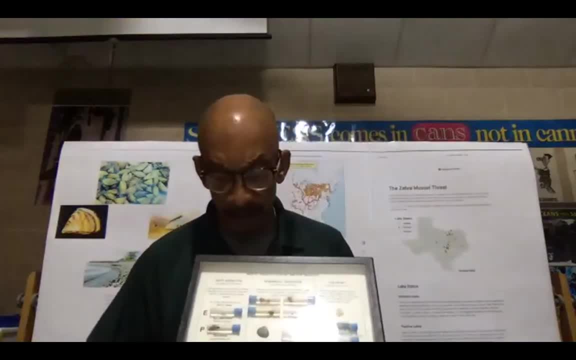 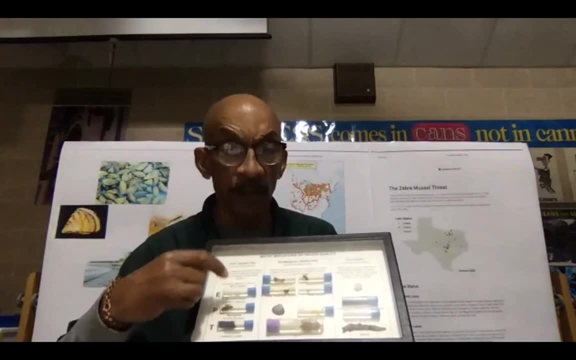 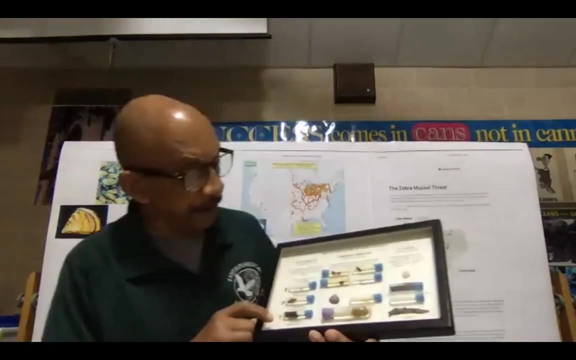 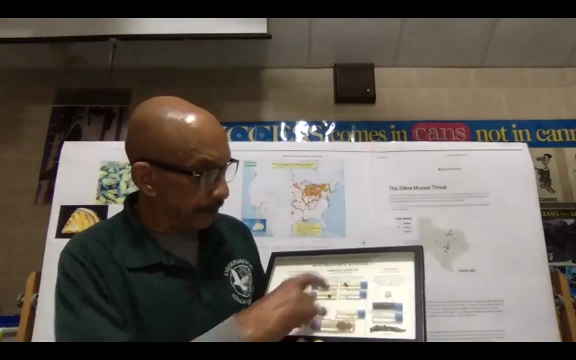 know whether you all can see this, but these are organisms, preserved organisms that are categorized according to how sensitive they are to the water chemistry in a particular water system, aquatic system. And this column here represents those organisms that are very sensitive, The middle column right here. they're somewhat sensitive. 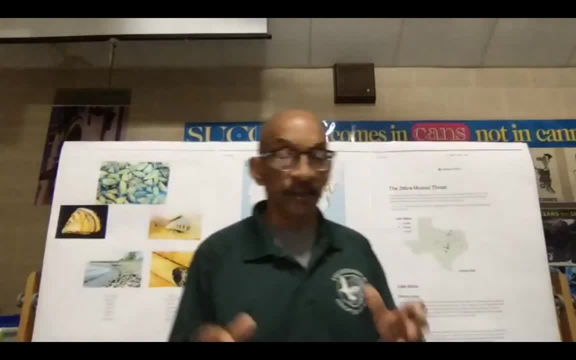 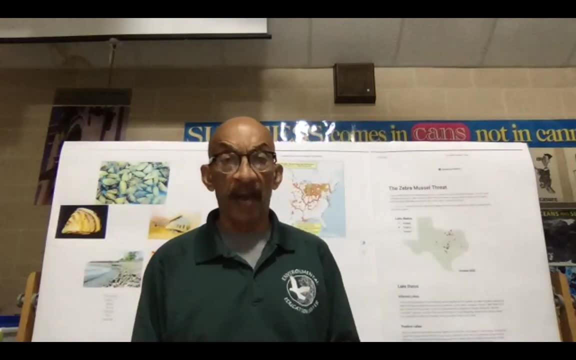 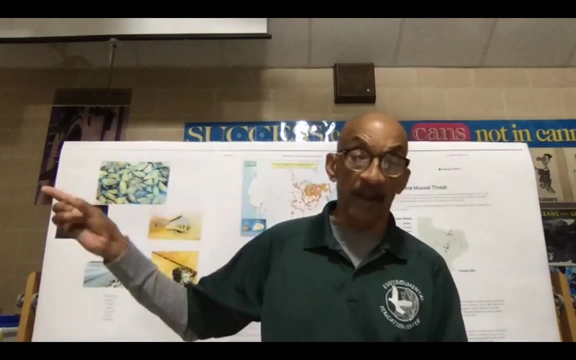 And one of the things out here that I realized over the years that I've been teaching here, that indicated that our ponds were pretty healthy, was the amount of mussels and clams that existed in those aquatic systems, Even in the big lake, Even in the ponds that have now gone dry. 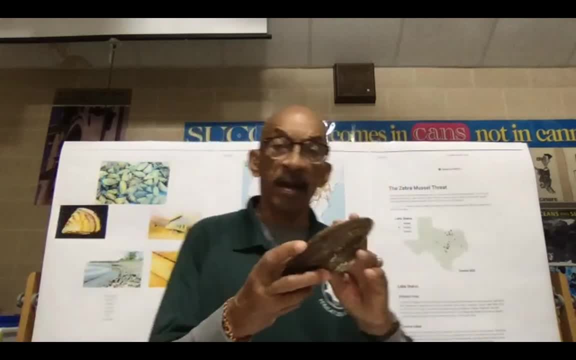 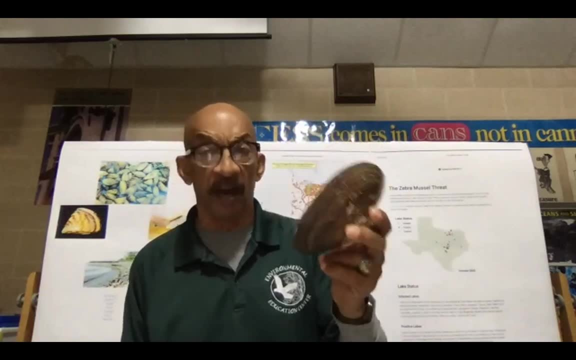 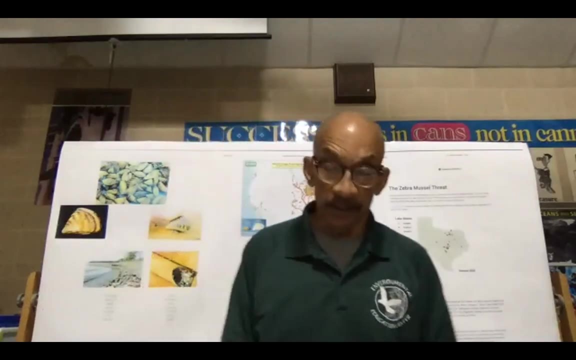 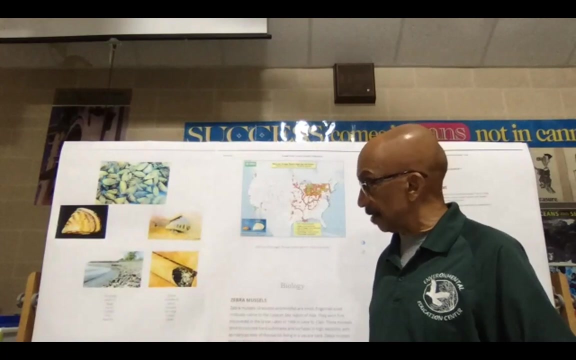 When those ponds went dry, we were able to find clams or mussels this size. So this mussel here has lived. it lived for a very long time And it indicated that the water quality was really good. Well, students, there is one type of mussel that is really invasive. 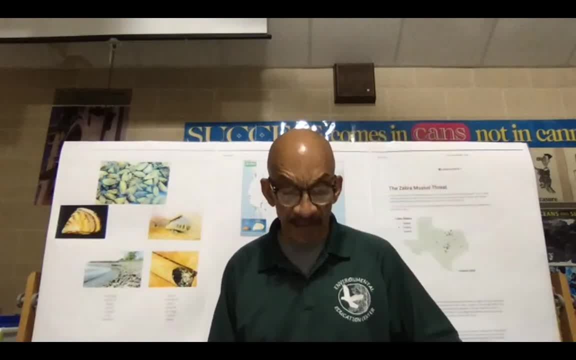 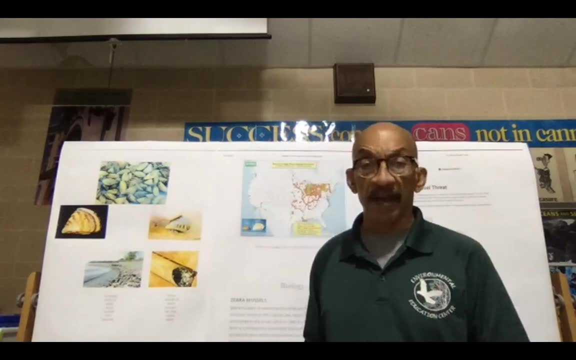 And it is a non-native invasive species. It is called Dracaena polymorpha And, in other words, the common name for that organism. it is called a zebra mussel. Now, how did the zebra mussel show up in? Texas. Well, it starts way back when ocean going boats or ships were built, And the reason why we have this species of mussel is because the ocean going ships came from Eurasia, Because this species of mussel is found around the Caspen Sea area in Asia. 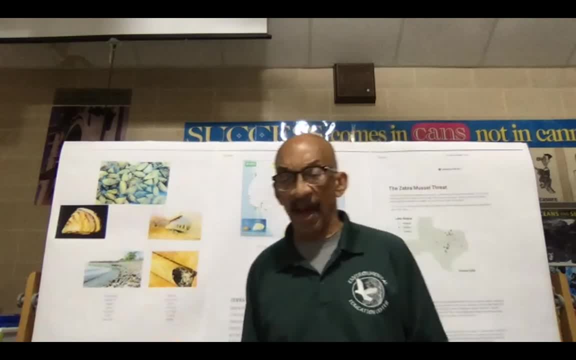 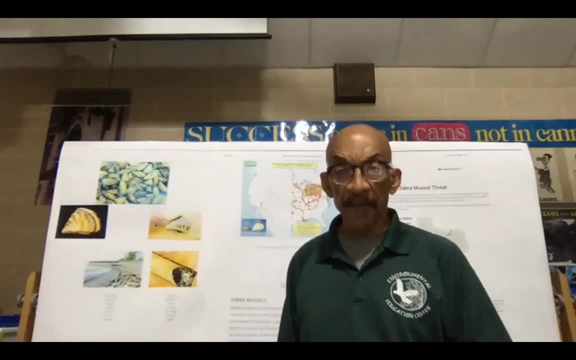 And it was brought here, brought to the continental USA, by ocean going ships that were loaded with ballast. Now, when we talk about ballast, that is the intake of water from a source and it's kept in the bottom of that ship or that boat to balance the boat and the sea. 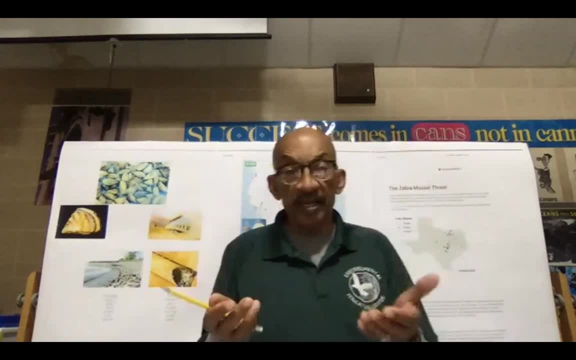 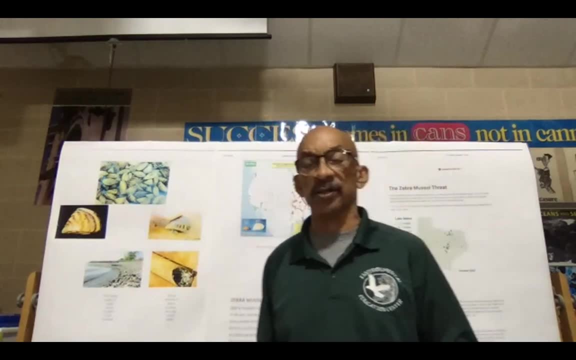 And that's where the mussel goes out. So it doesn't lift to one side or it sets at a certain level in the water. Even with some of the boats that we use for fishing today- bass boats and ski boats- there's a certain 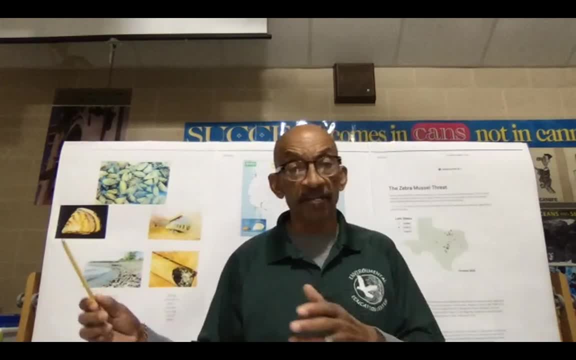 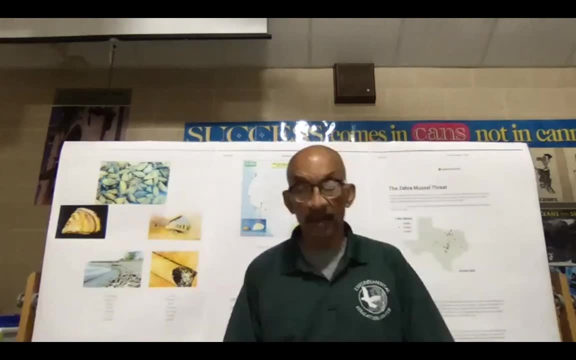 amount of water that is taken in. Well, anyhow, these ships came across from Eurasia and they entered the Great Lakes, because in 1986, that's when they were first discovered in the Great Lakes, in the lake of St Clair- Now these mussels colonize. 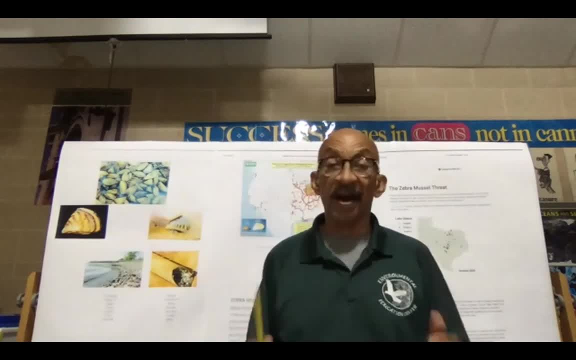 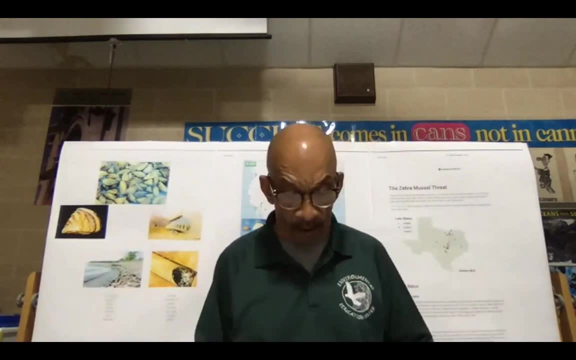 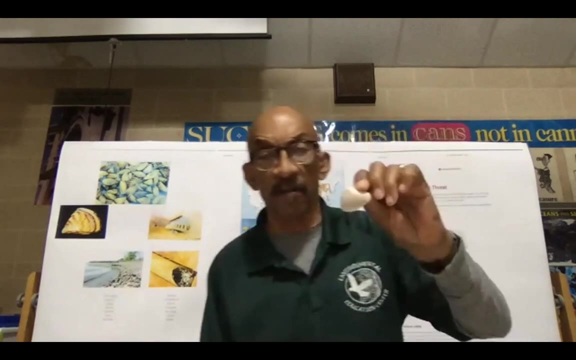 on hard substrates and surfaces in high density. As many as tens of thousands of these can exist in a square yard. They're about as big. a large one would probably be about as big as my fingernail. This is very similar to a zebra mussel. 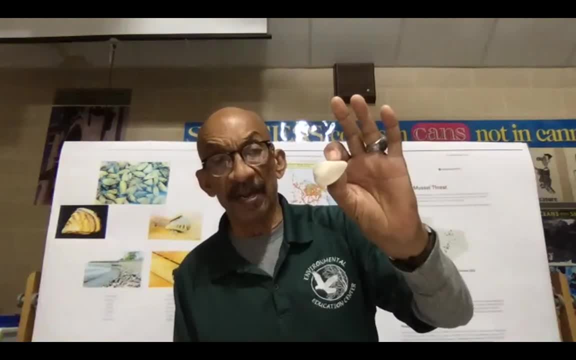 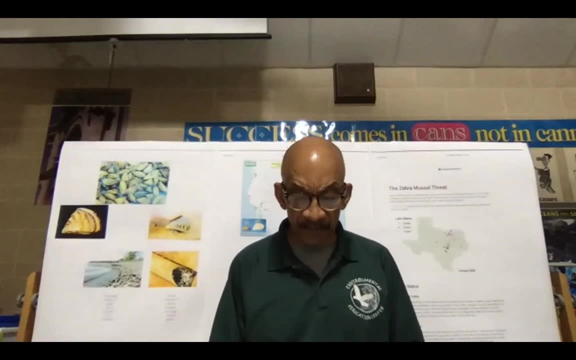 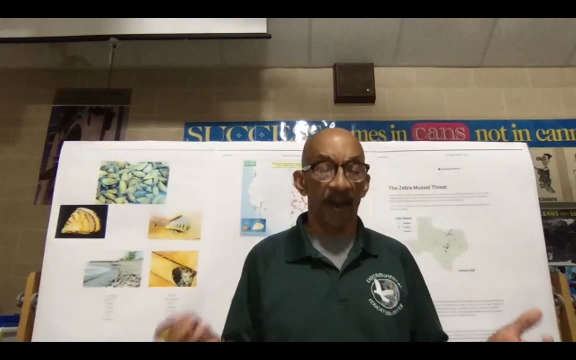 but it's not. Zebra mussel would not be quite that large, very small. And the thing about the zebra mussel: they feed by filtering water to collect phytoplankton, where the phytoplankton is clinging to substrates. What happens with the zebra mussel is: 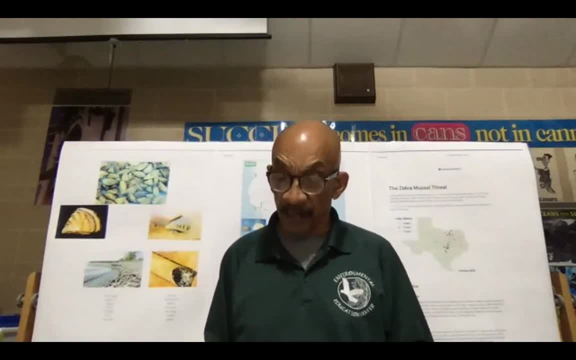 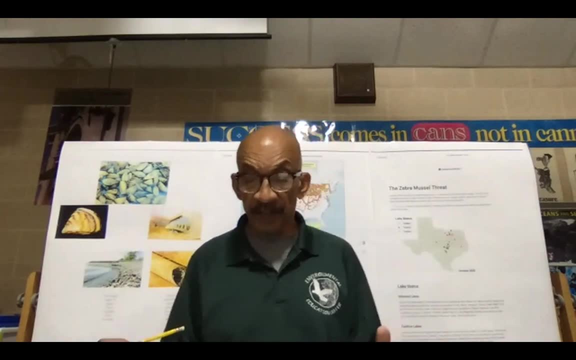 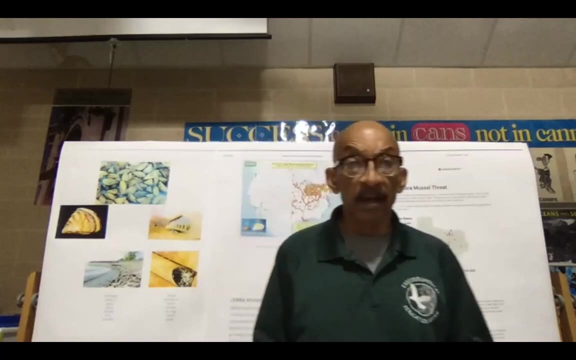 that they reduce the amount of phytoplankton that's available for other organisms and they increase the water clarity, thus changing the structure of the local aquatic communities that we have around. Now that zebra mussel occurs in three different stages. 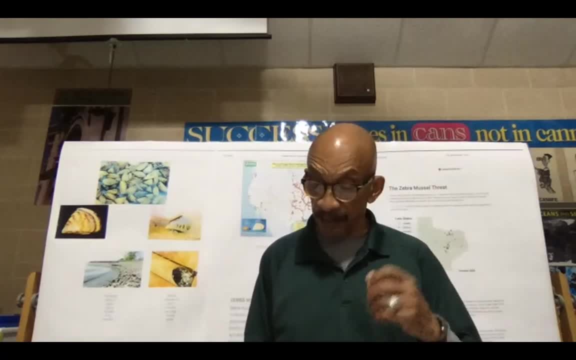 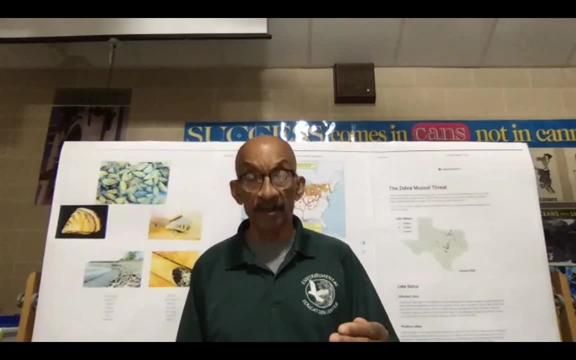 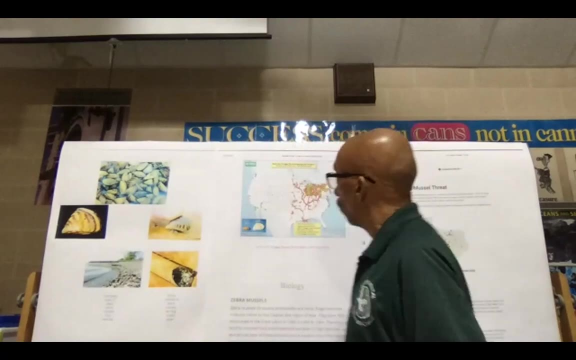 The larva stage, the juvenile stage and the adult, And basically they are transported to new ecosystems via currents and ballasts And they can stay alive for several days without being in water. We look at this map here. in fact, I'll. 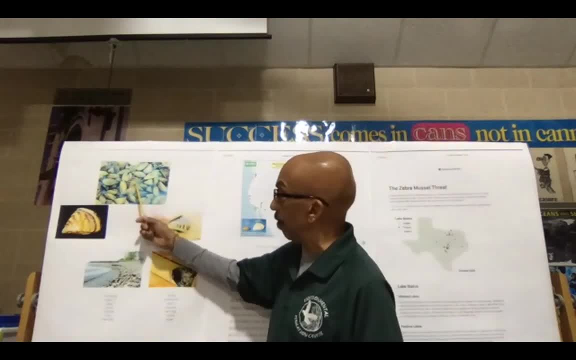 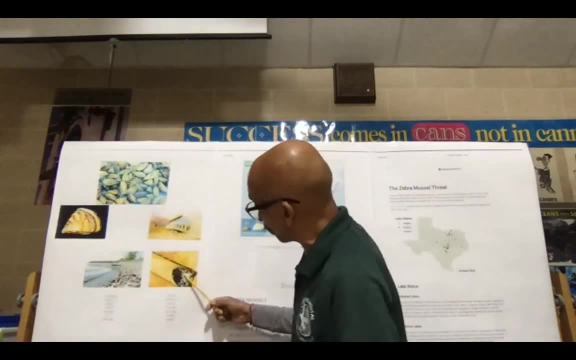 go back over here, And this is the description of what a zebra mussel would look like. They have stripes, and that's probably how they get their common name. In this picture you can see that there are hundreds of them clogging up this section of pipe that was taken out. 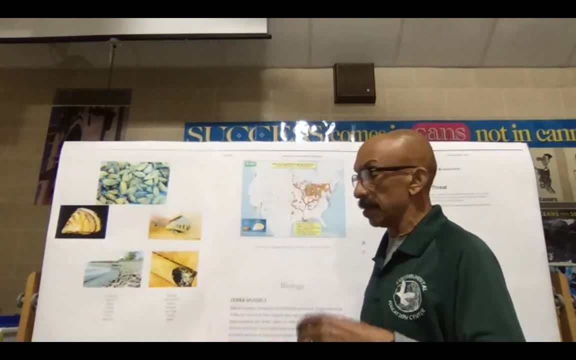 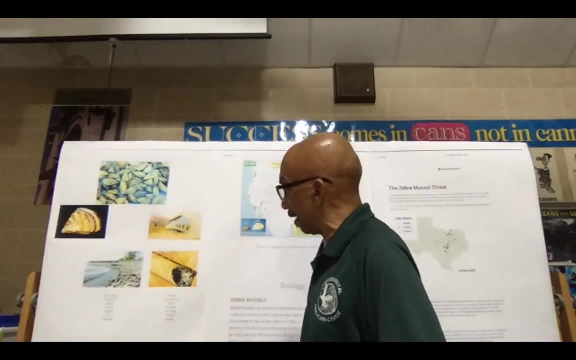 So what that means is they can clog up industrial pipes, power plant pipes, all those pipes that use water as an intake to disrupt even the power plant, And that's what we're getting from power plants Along this shoreline that we see here. there are thousands upon thousands. 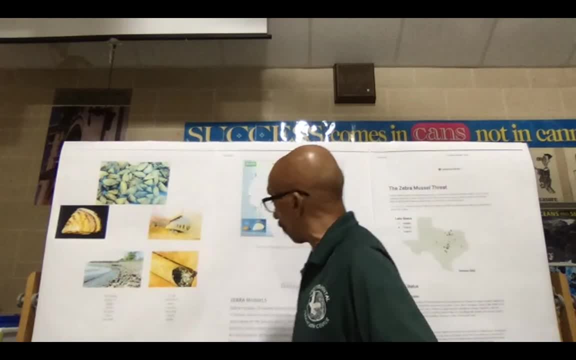 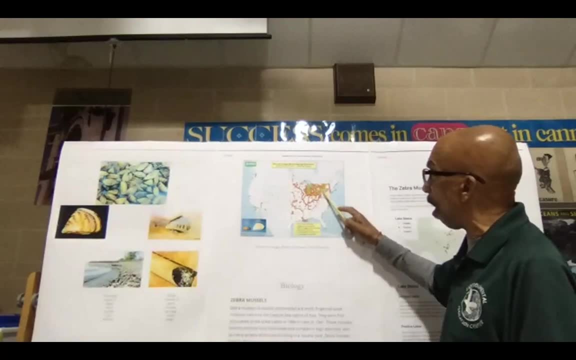 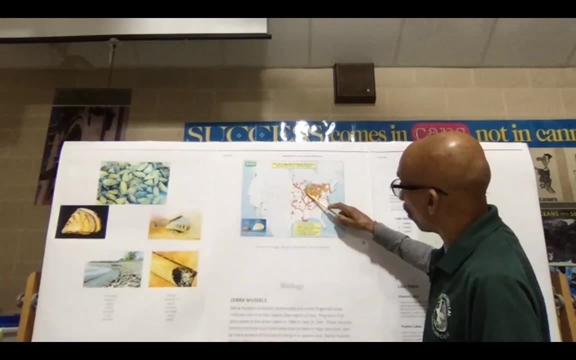 of dead zebra mussels, So they are a very big problem Now. they started out in the Great Lakes. In this map here we see all this orange. There is some green which represents other types of mussel occurrences, But where you see the orange. 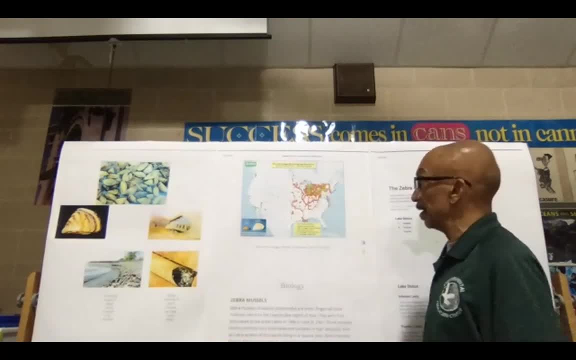 that's where there has been evidence that zebra mussels are there. Now, as you look down toward Texas, we have them in Oklahoma, we have them in Kansas, we have them in Arkansas, right down through and even down the Mississippi River. 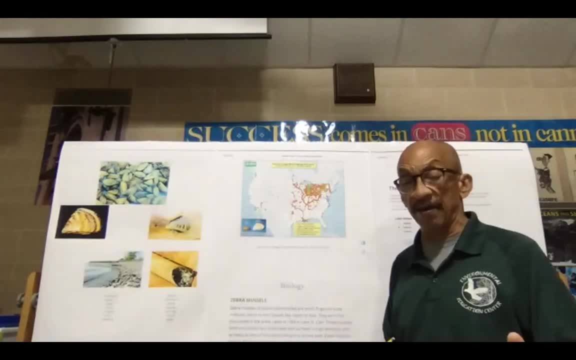 So they do flow with the current. They not only can be found in an elliptic body of water, which is still water, but they can be found in an elliptic body of water, which is flowing water. When we look at the state of Texas. 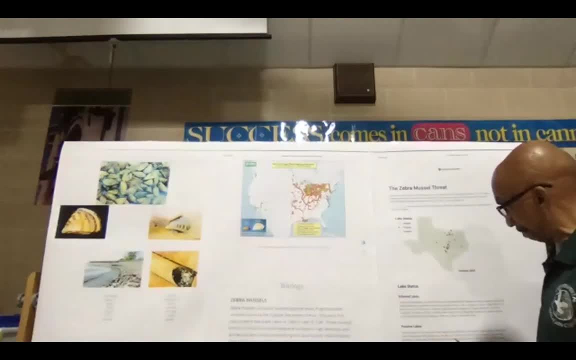 there are a lot of lakes, of what we call infested. There are some lakes that are what we call positive. Now, when we talk about infested, we're talking about they have a big population that has been established and they are now considered to be a reproducing population. 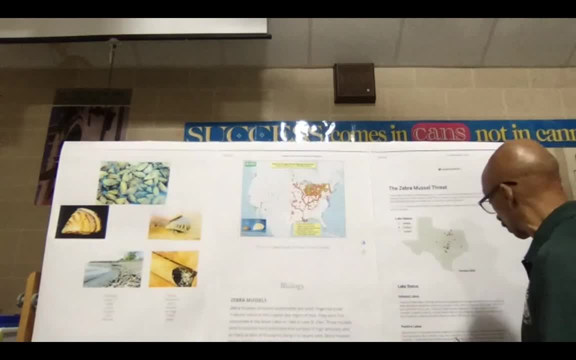 And I'm going to name some of the lakes, and some of you may be familiar with some of these lakes: Lake Austin, Belton, Bridgeport Canyon Lake, Dean Gilbert, Eagle Mountain Lake, Georgetown Lake, Granger, Lake, Grapevine. Ladybird Lake, Louisville Lake, Livingston Lake, Lyndon B Johnson Lake, Marbles Falls Lake, Pflugerville Lake, Fluderville Lake, Randale Lake, Lake Ray Roberts, Richland Chambers, the Steelhouse Hollow Lake, Lake Texoma and Lake Travis. I have fished some of those lakes. 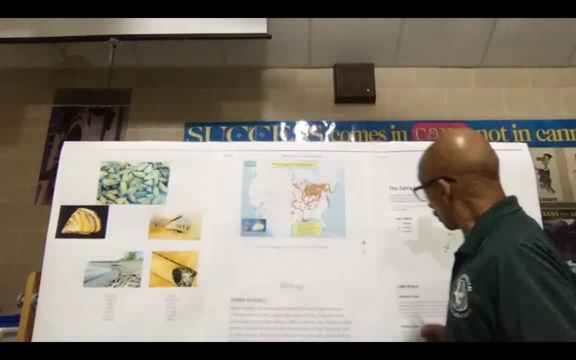 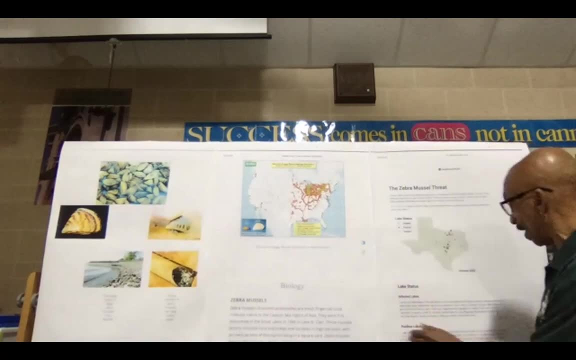 but that's been some time ago. These infestations are probably the most recent infestation. okay, Now there are a list of other lakes that are considered to be positive, And I will tell you. I see one river that has been deemed positive. 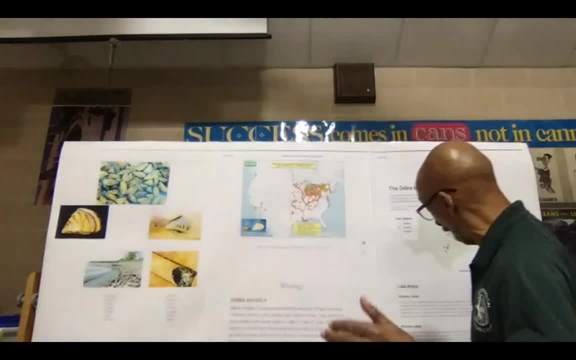 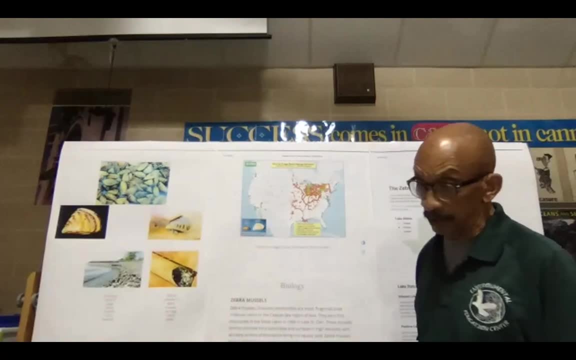 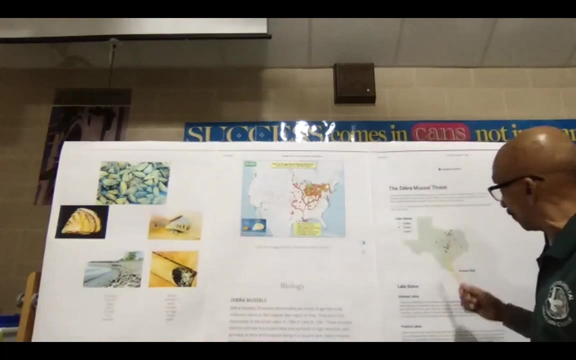 and that is the Trinity River, which runs right through Dallas. So these mussels are very intrusive, very invasive and they can cause a big problem students. One of the things that Texas Parks and Wildlife have done is that they have created a monitoring system. 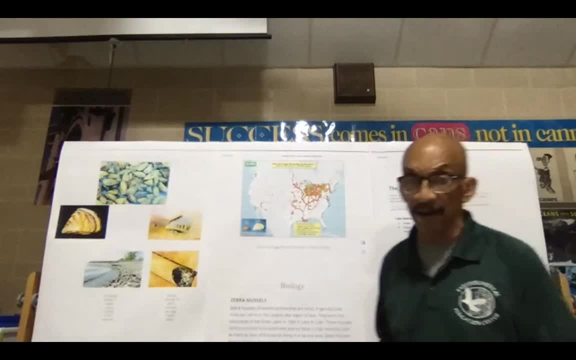 to monitor and to test and they've given a hotline. You can go online and you can find that hotline if you find evidence of the zebra mussel. They also now have new regulations that they're warning boaters- anybody that's using water. 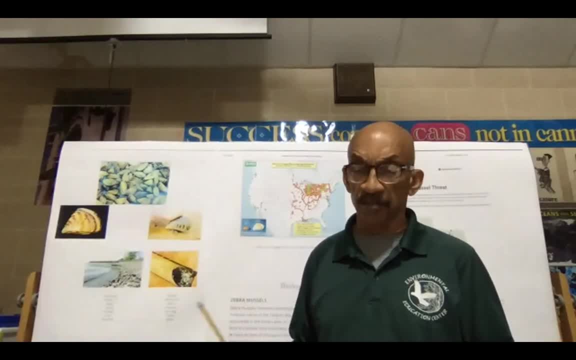 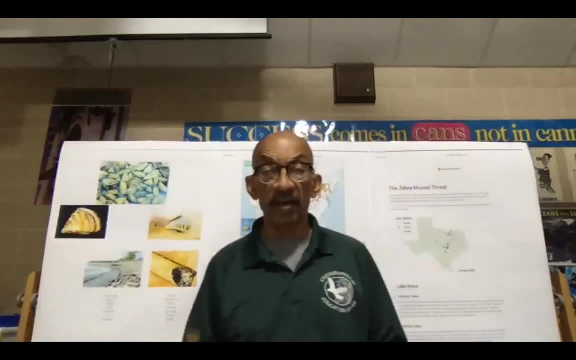 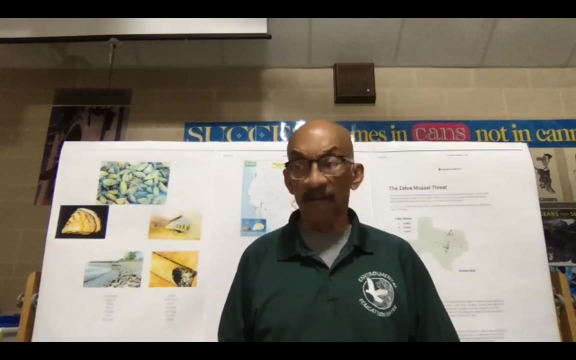 that's using water out of a lake to for recreational purposes- boating, ski boats, all that fishing. they're now requiring that when you leave that lake, you empty all the ballast that's in your boat, even the log wells that you're keeping your bait. 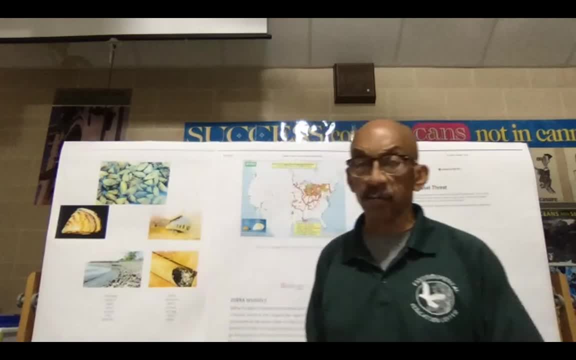 or your fish in your bait buckets. You do not transport any of that lake water to any other public water areas simply because they're not in the water. Because, remember, these zebra mussels can stay alive three days without being in water. 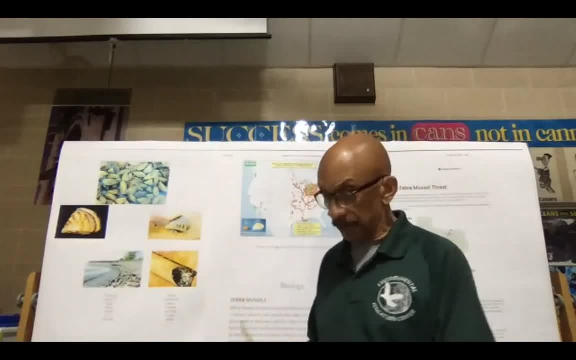 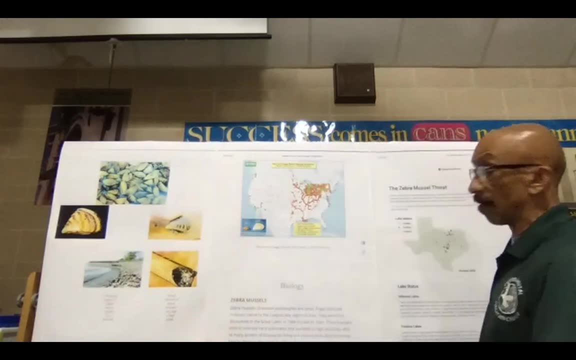 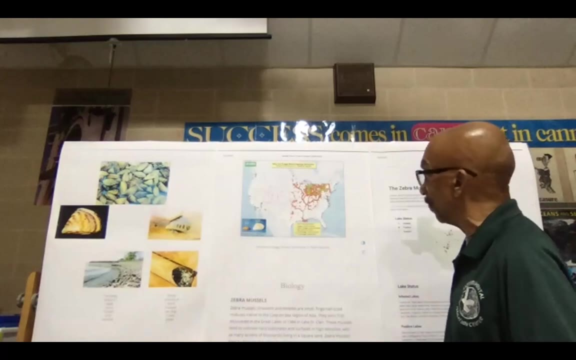 So that's what makes them and they can attach themselves to boat motors, the underneath sides of boats. They have a very high survival. I call it survival skill. They're gonna survive wherever they can cling on to and move themselves to. So it is said that possibly if you're caught, 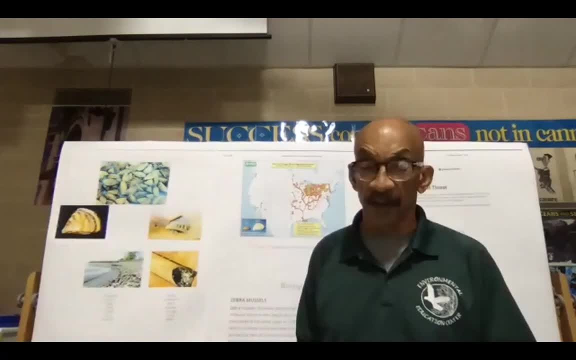 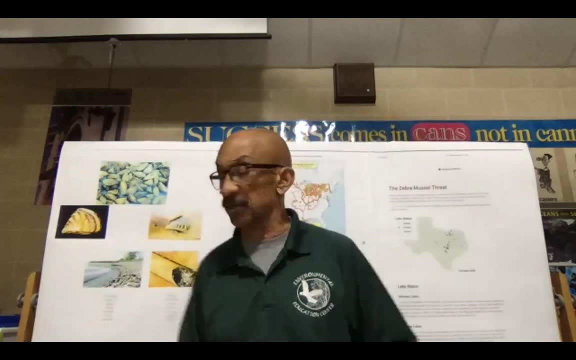 transporting these guys, whether you're doing it on purpose or not. you can be fined up to $500 per incident. So it's better to be safe than it is to be sorry. And these numbers are actually. believe it or not, these numbers are growing. 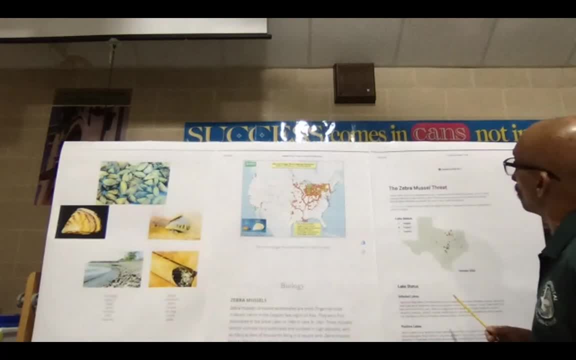 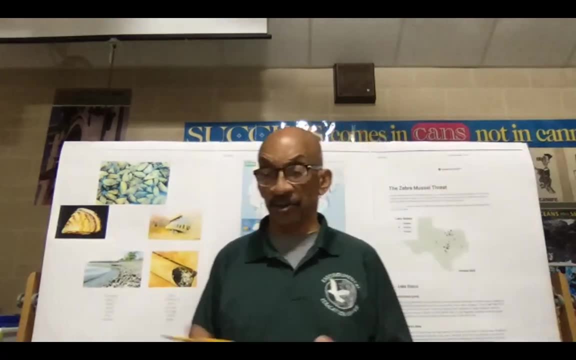 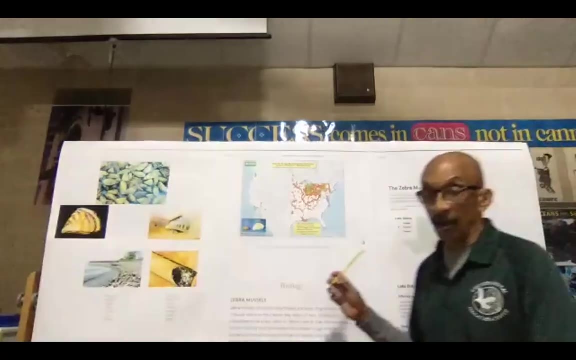 This was the last count and this was taken the first part of October. So when spring comes, when summer comes and there's lots of people on the lakes and stuff, we need to really be visual in following those guidelines that Texas Parks and Wildlife have put out. 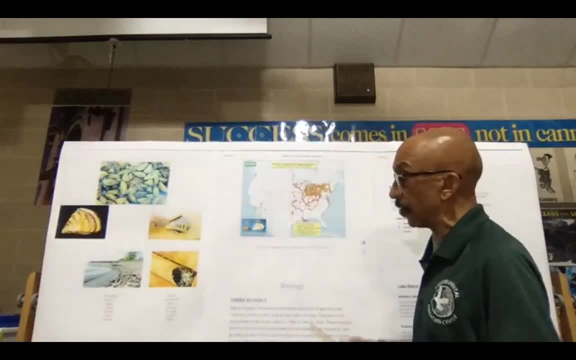 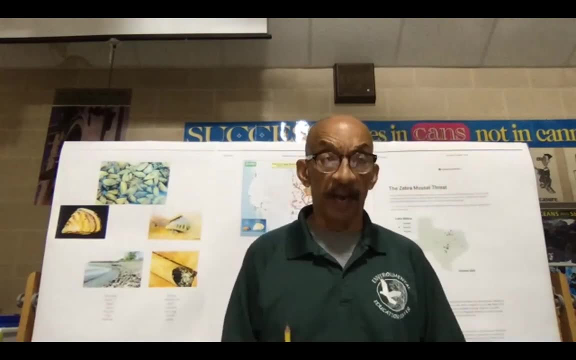 Because, again, not only are they affecting the life that's already established in that ecosystem, they're also affecting your daily life by cutting down on damage to power plants or increasing or doing damage to power plants. Even the water that we consume in our everyday lives come from those reservoirs. 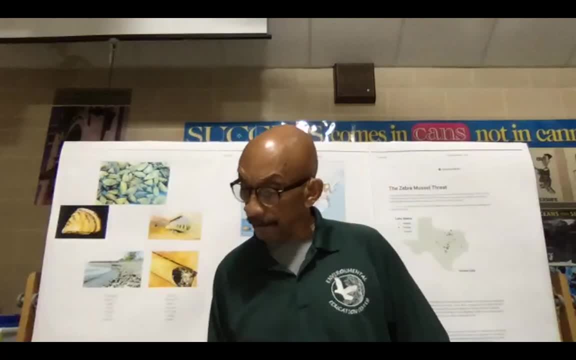 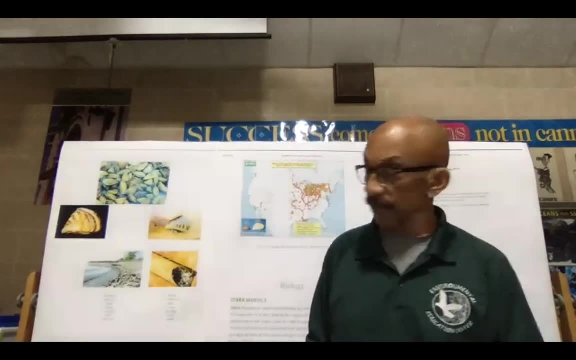 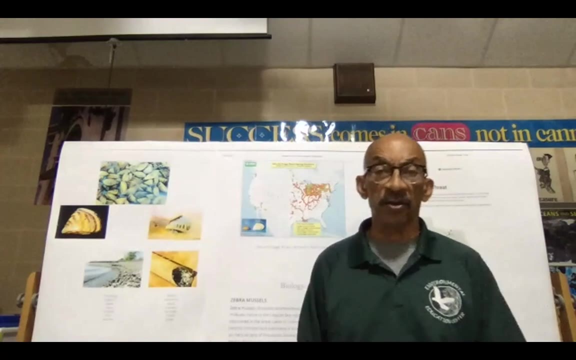 like Ray Roberts. In fact, that was one of them that is infested, And I will share this with you. I forgot to tell you that the first ones that were discovered here in Texas, they were discovered in the year 2009.. 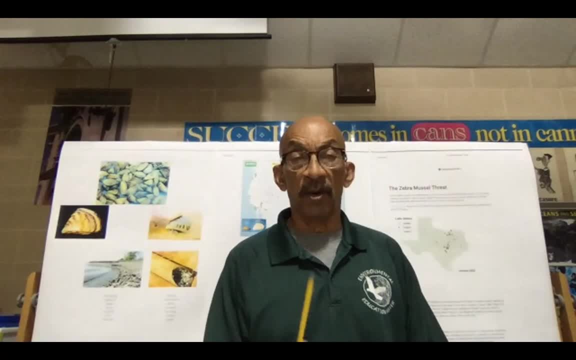 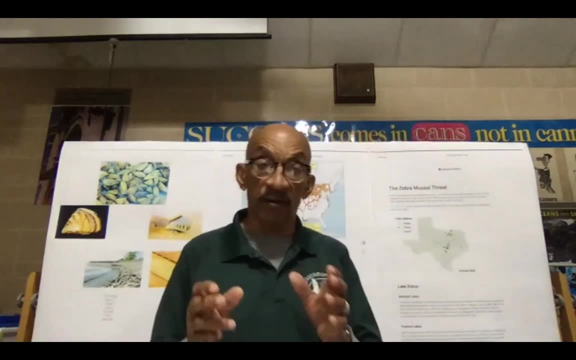 And that was only one lake that had them at that time, And that was Texoma Lake, Texoma. So that is an example of how humans had contributed to organic problems with our ecosystem, And those organic problems stem from the zebra musk. 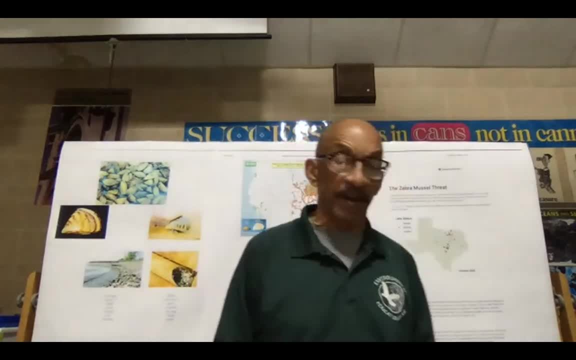 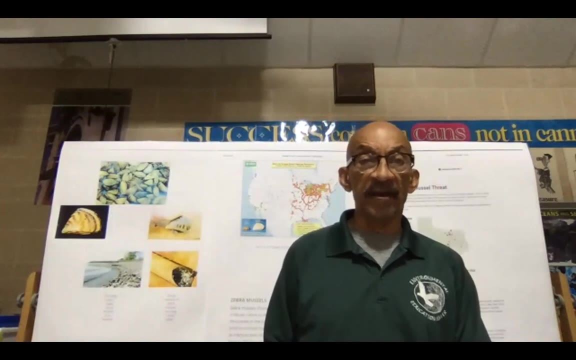 Hopefully, I've been able to give you a little good information about an organism that has indeed grew out of proportion simply because of human aid, human health And our unawareness. I want to thank you for your time And, guys, I want you to have a good rest of the virtual field. 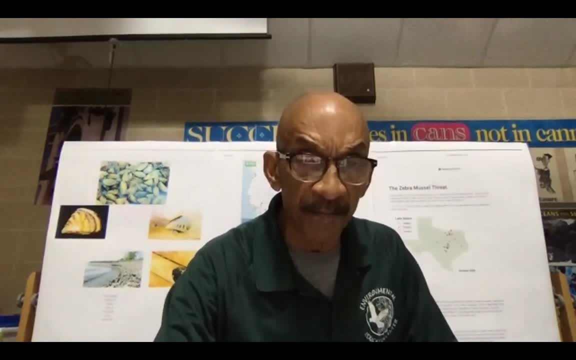 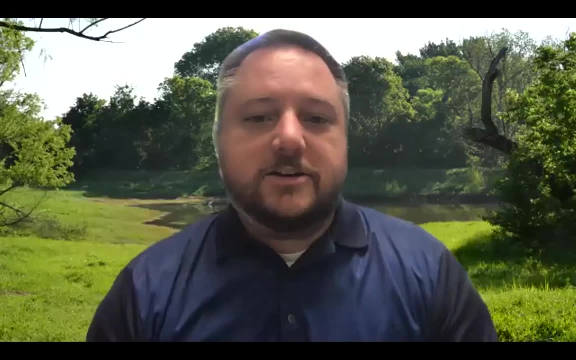 trip today And I'm going to turn it back to Mr Broaden, in case some of you have some questions you want to answer. I'll see you later. Thank you, Mr Monroe. We got two questions. The first question was: do we use clams here? 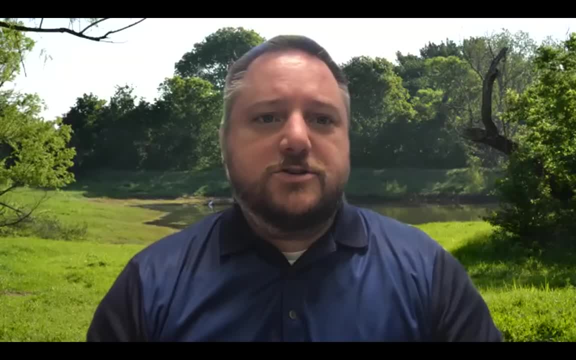 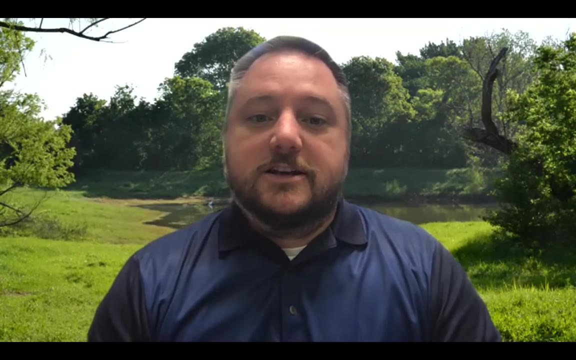 at our environmental education center- And yes, we do. We have a living materials center that we send out fish to teachers from, and sometimes put clams in those aquariums because they are an indicator of healthy water. So you can kind of just if the clam is doing well. 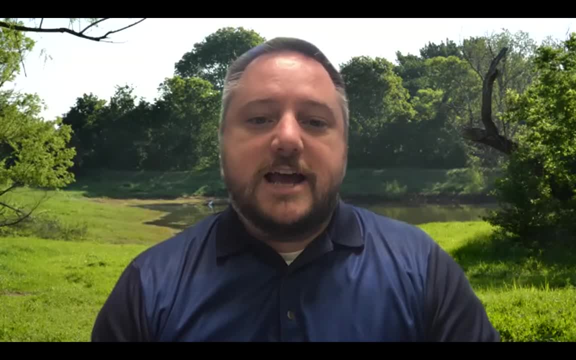 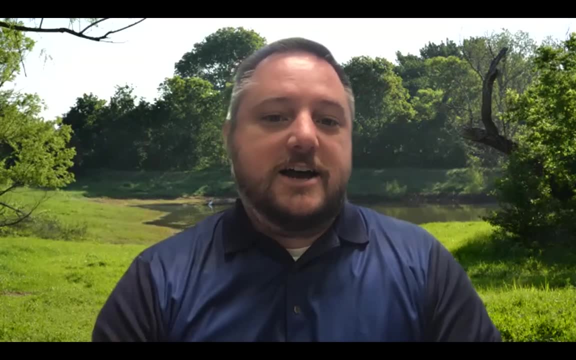 you know the water is healthy without having to test it. And then the other question was: do we have any zebra mussels? No, we do not. Those are illegal to possess. So we don't have any here And we don't want any here either, because they are invasive. 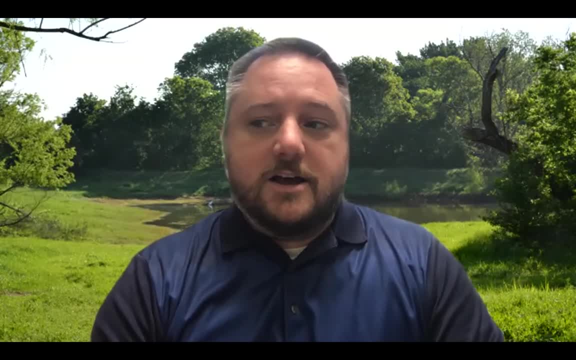 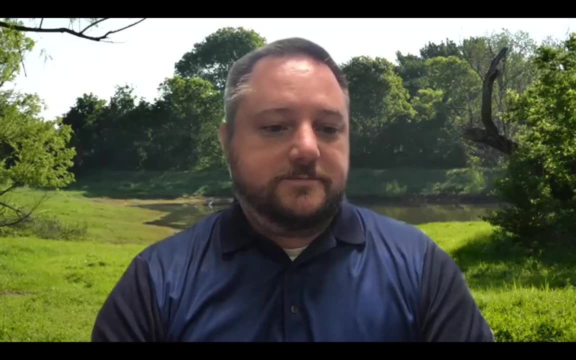 and can mess up your ponds or lakes. All right, Now we're going to move on to the The effects of physical changes on aquatic ecosystems with Mrs Fuller. Good afternoon, boys and girls. We're going to look at a big word: anthropogenic. 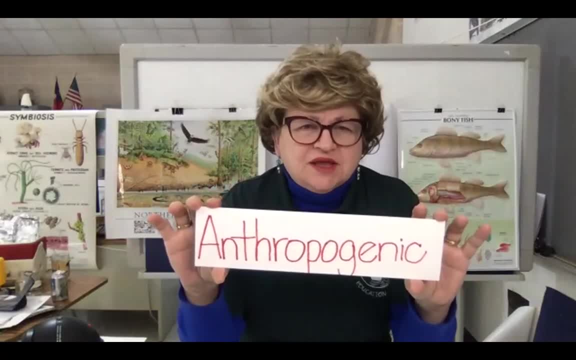 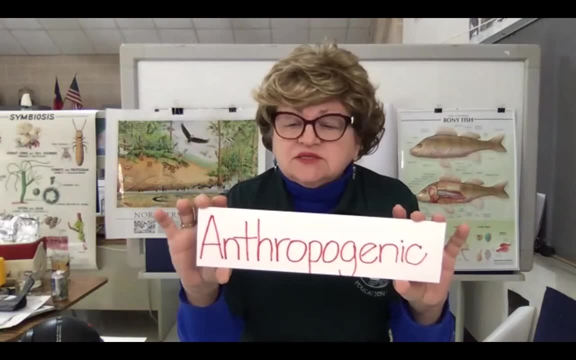 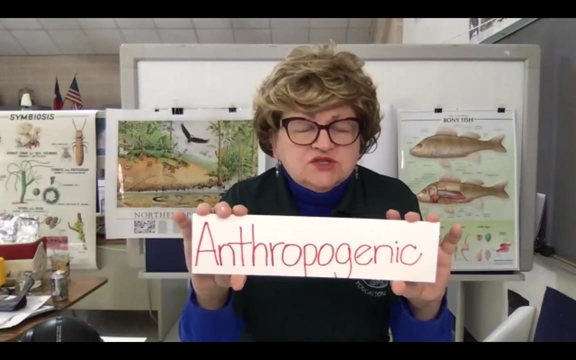 And what that means is originating in human activity, Essentially means caused by mankind, And this segment will cover human aspects of the physical part of the freshwater ecosystem. Now, like Mr Monroe pointed out to you, the two different kinds of freshwater ecosystem are Lodic and Lintic. 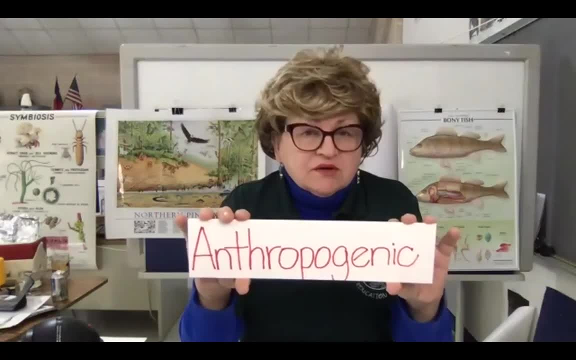 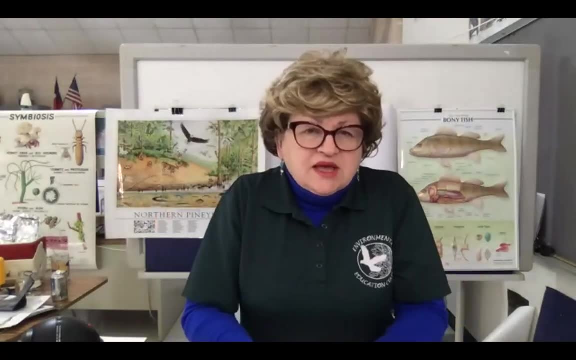 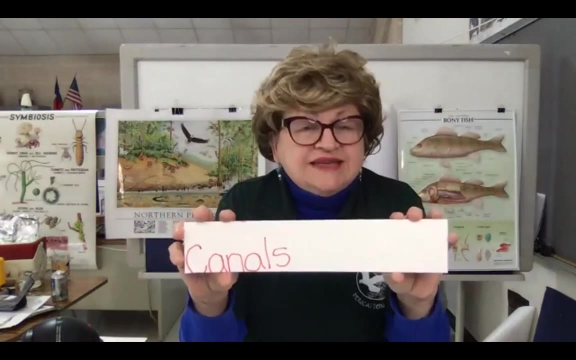 Lodic means flowing, Lintic means still water, like lakes. So we're going to start off with the Lintic aspect and talk about five really big lakes at the top of the United States: the Great Lakes In the late 1830s to early 1840s canals. 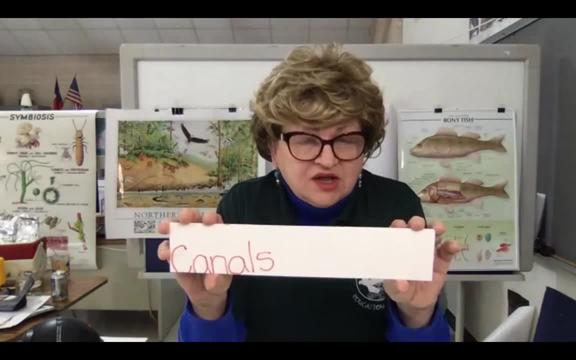 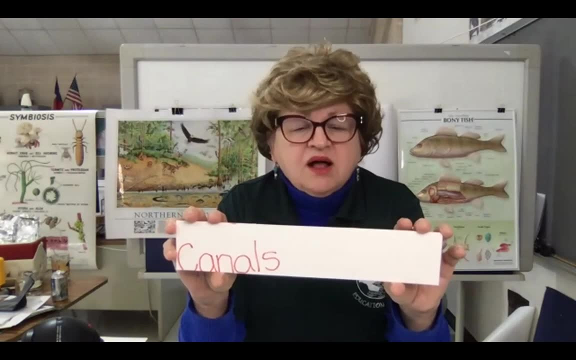 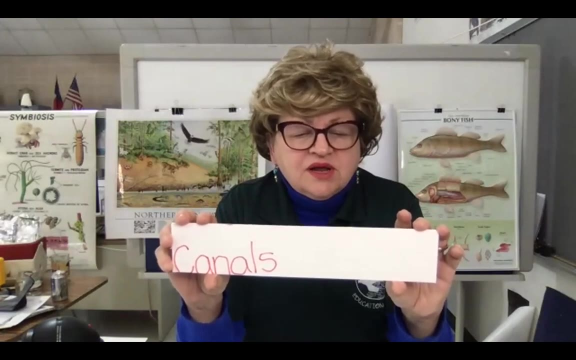 were dug to connect the Atlantic, Atlantic Ocean to the, to the lakes, And this was to transport goods, to transport people, all sorts of products, all sorts of things like that, And the Great Lakes are Ontario, Erie, Huron, Michigan. 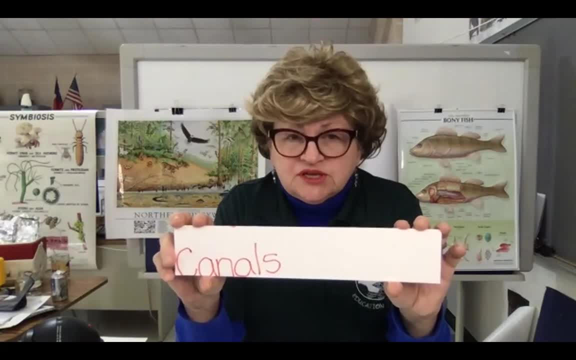 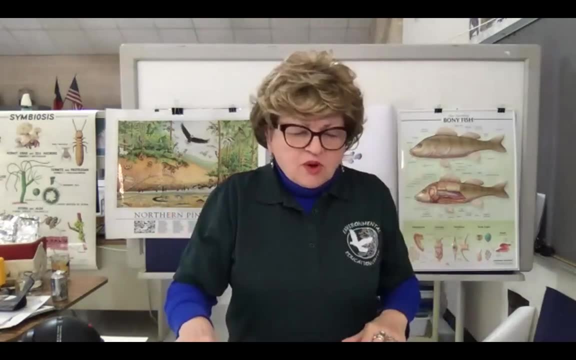 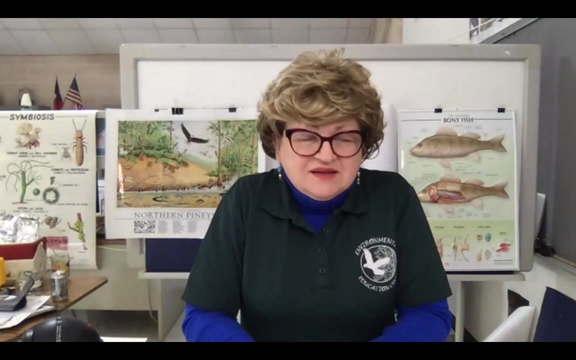 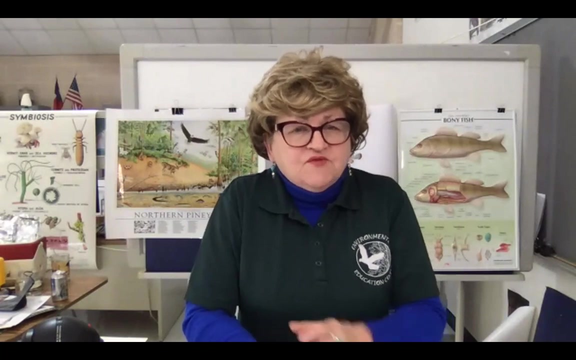 and Superior, And they hold 21% of Earth's surface freshwater. So this is a tremendous amount of water. Well, these canals that these People 100 and something years ago dug, almost 200 years now. their purpose was to make things easy for people and stuff. 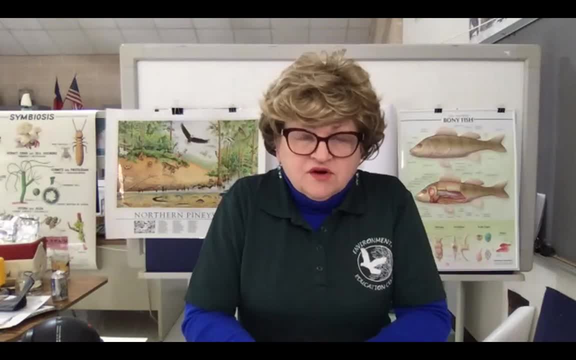 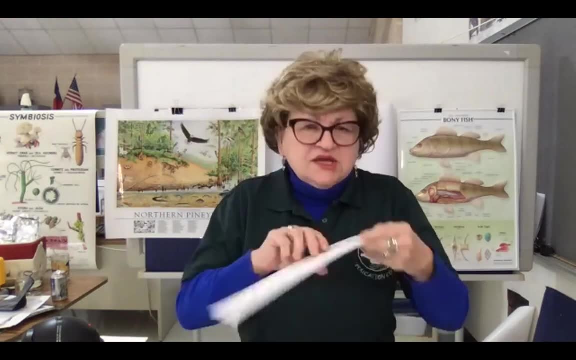 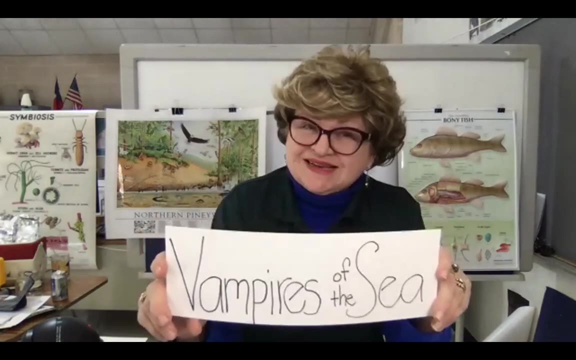 to get from one place to the other And it worked, And it worked very well. But it had an unintended consequence, And that is it: allowed into the Great Lakes. vampires- They're called vampires of the sea. That's their nickname. That's not the real name. 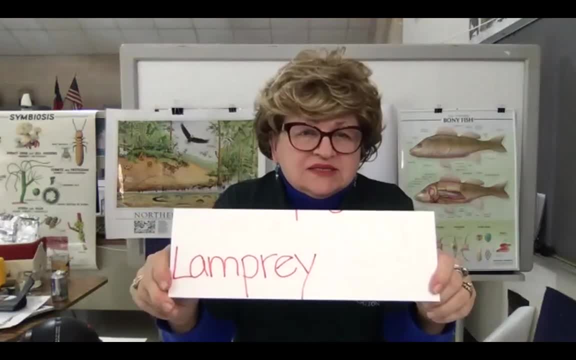 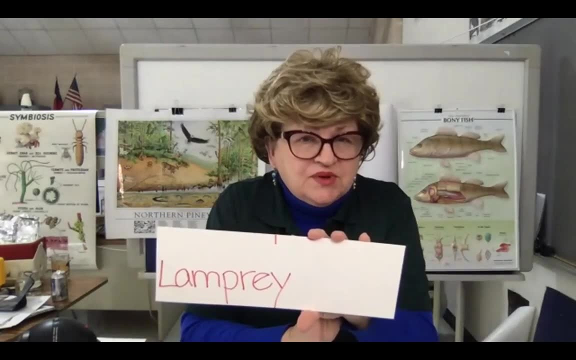 The real name is the lamprey. The lamprey is a very, very ancient fish. It's a jawless fish, It's cartilaginous. It's not a bony fish And it doesn't because it's jawless. 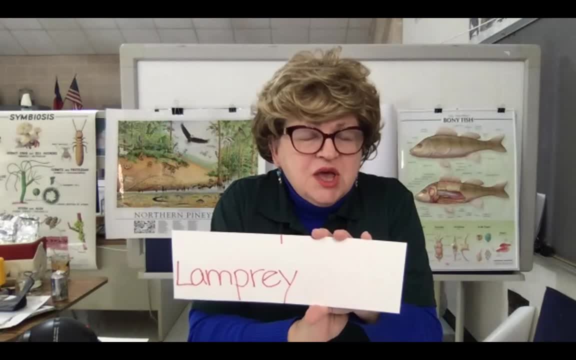 it doesn't have a proper mouth that you would think of for a fish, but rather has a circular, raft-like mouth that he attaches to the side of fish and he sucks out the fluids from the fish Over the course. he's usually an adult for about six years. 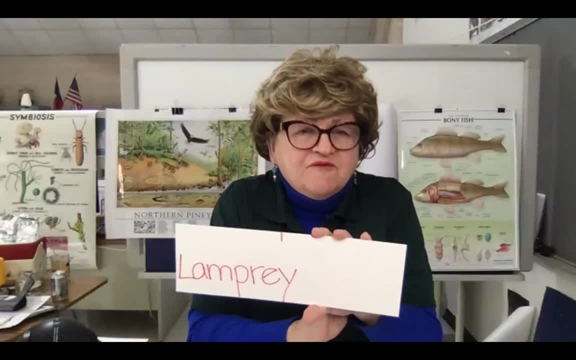 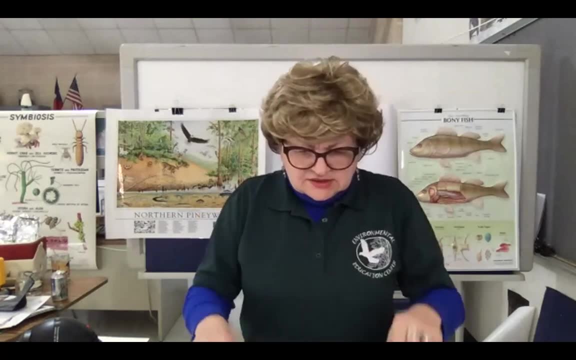 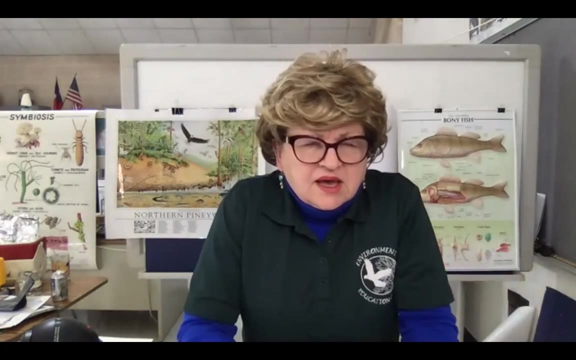 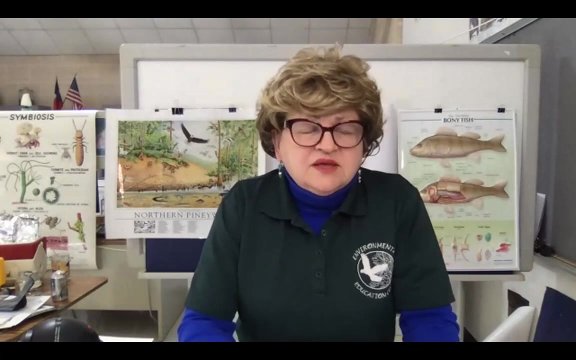 And over the course of those six years he will consume about 40 pounds of fish, flesh and fluids. All right, So what has happened is the Great Lakes used to be a huge source of food fishing. The fishing industry was enormous in the 1800s. 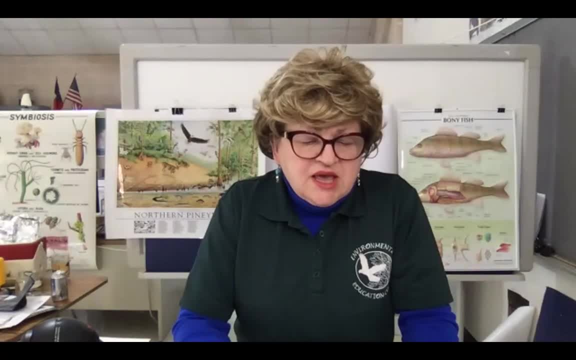 and the early part of the 1900s In Michigan, Lake Michigan- in 1946, 5.5 million pounds of fish were caught And by 1953, they caught 402 pounds, Not 402,000, 402 pounds of fish. In just that short time. So it's really sobering. Lake Huron went from 3.4 million pounds of fish in 1937 to zero in 1947. So within 10 years the Lamprey had completely decimated the fishing industry in Lake Huron. And it got to Lake Superior. They attached themselves to fight trout, all kinds of big fish, And they have no natural predators because they didn't evolve in the Great Lakes. They evolved in the ocean where there were predators, But this parasitic fish has just devastated both sport fishing. 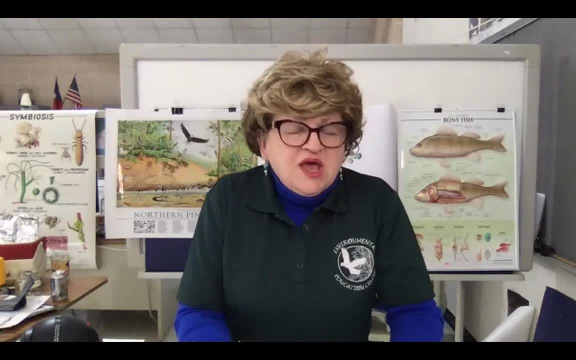 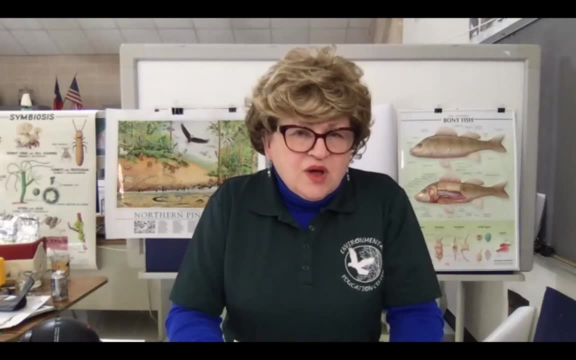 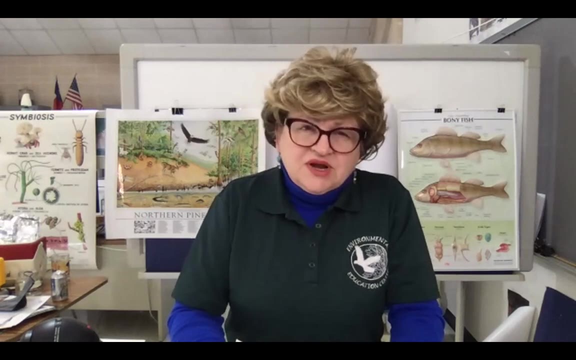 and the fishing industry for food in the Great Lakes, And they had spent about $20 million a year trying to find different ways to get rid of the Lamprey, or at least hold it. So it started out as a really good idea to change the physical environment of the lakes. 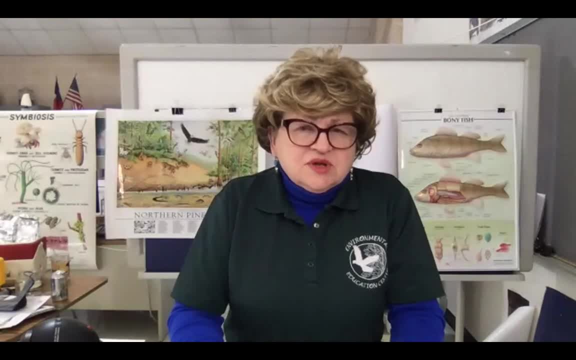 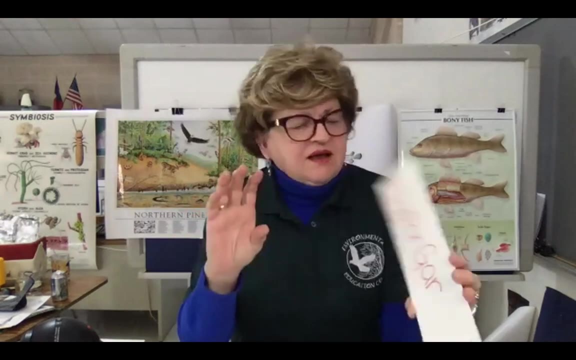 by building canals, But it ended up being just completely destroying the billion dollar fishing industry. Now let's go to some Lodic water. All right, Here in Texas we've got a guy called the Alligator Gar, And he is also a very ancient time. 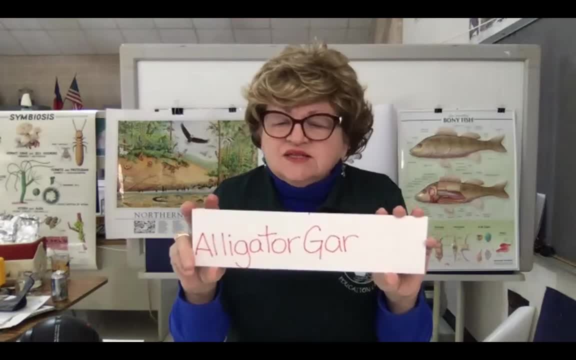 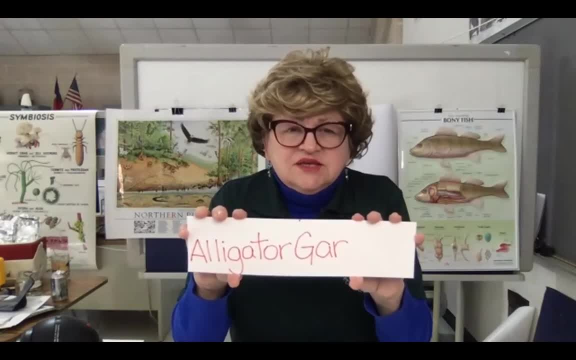 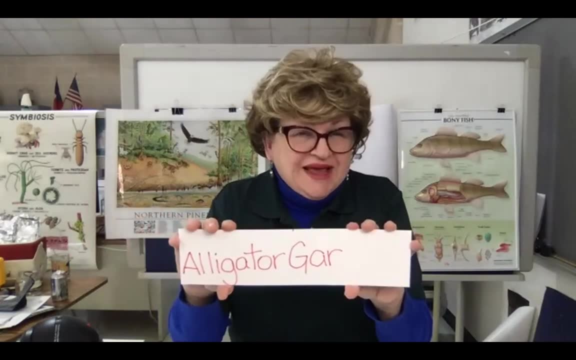 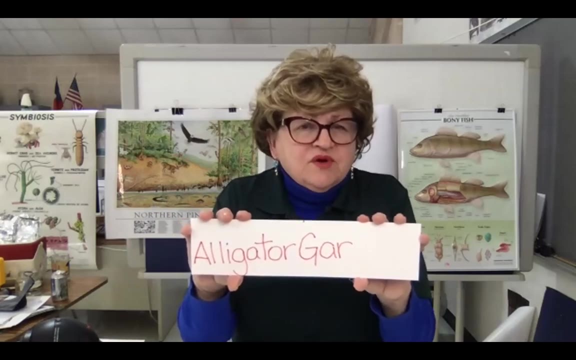 But the way they lay their eggs is: when there are seasonal floods and the floodplains get flooded with the monsoon rains, they go out into the floodplains to lay their eggs. They don't lay their eggs in the river bottoms themselves. 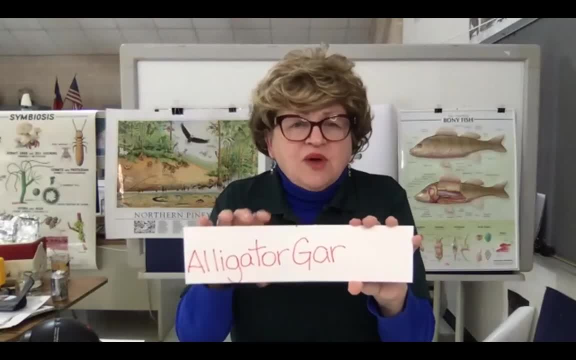 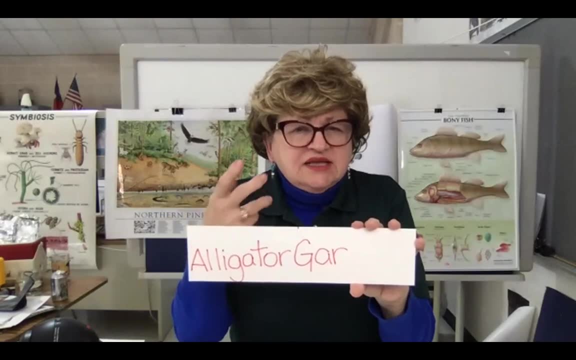 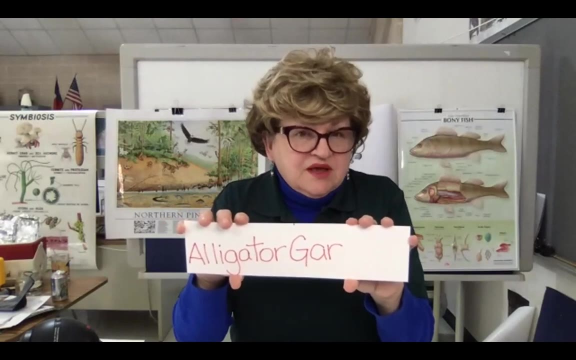 or in the river bank themselves. They go out into these floodplains and they'll stay flooded for several days, And the sticky little eggs will attach to some plants, They'll become larvae and then they'll become fry, And by this time they're big enough to avoid pressure. 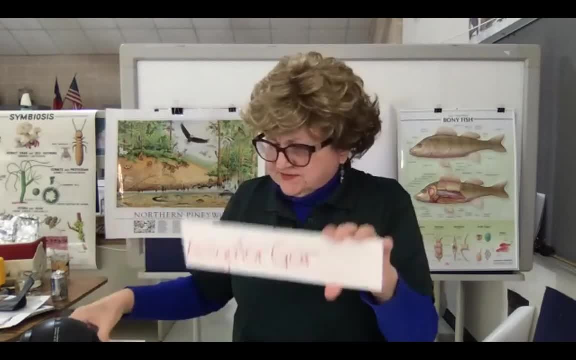 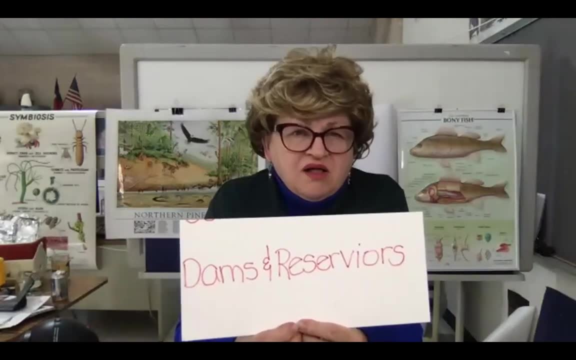 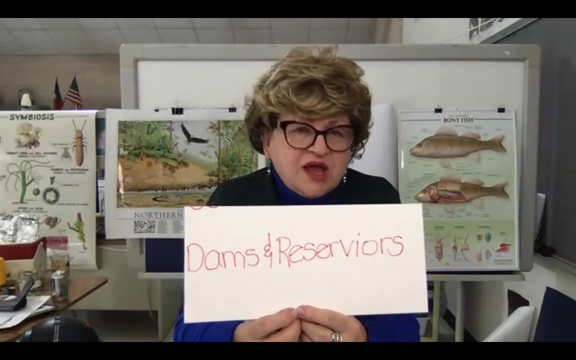 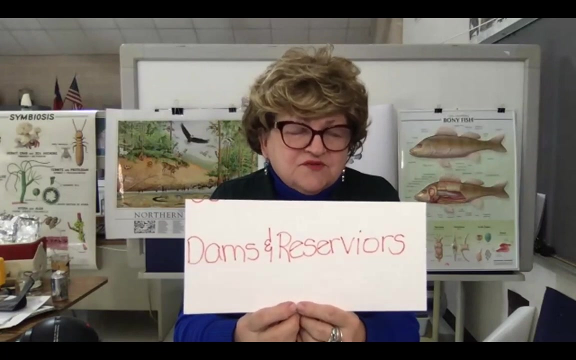 They're not predators. Well, human beings, in these great ideas, have built dams and reservoirs along all the rivers. That's the loaded water, That's the water that flows, in order to provide recreation and flood control and all kinds of different reasons why we build reservoirs. 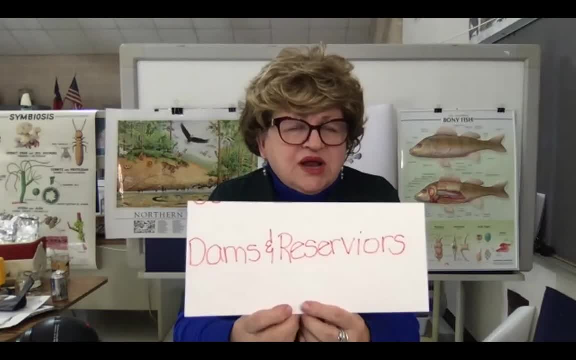 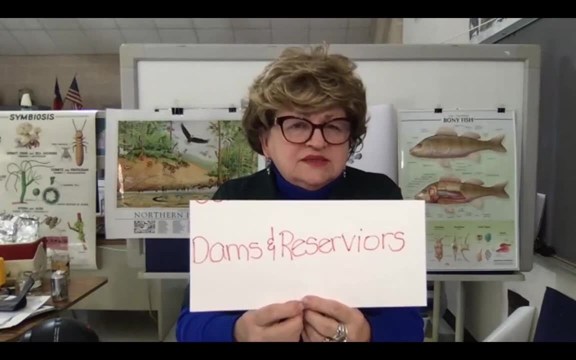 drinking water and that sort of thing, And that's a really good idea for humans And it's a good idea as far as protecting cropland from floods. But by this water management they've also eliminated these seasonal floods and have eliminated the opportunities. 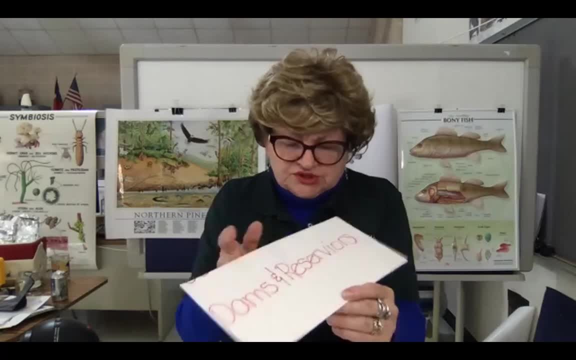 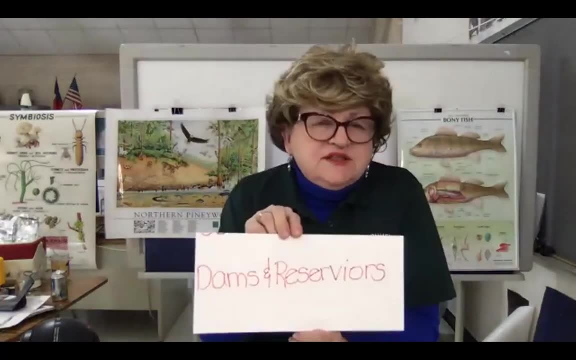 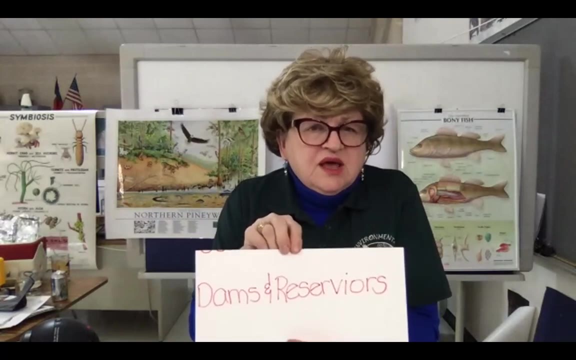 for the alligator gar to reproduce. The alligator gar has other problems besides these physical changes that humans have made in their environment. They've suffered habitat, habitat loss, overfishing. for a long time They were considered a trash fish and people would just kill them willy-nilly. 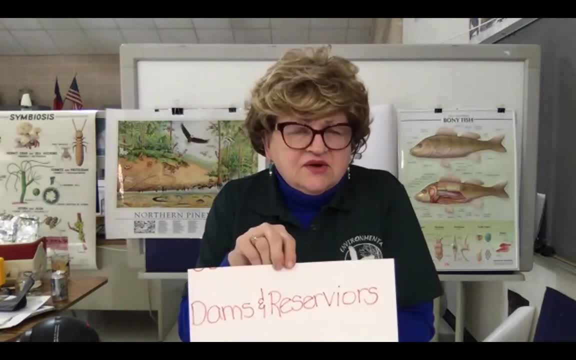 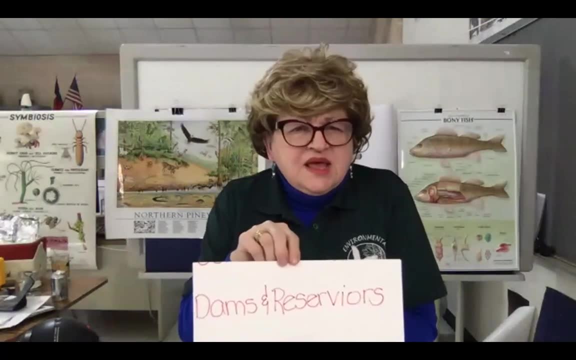 There are people who like to eat the meat of the alligator gar. It's got a very firm flesh. It's not flaky like flounder or trout or anything like that, And they've got a very unusual scale. The scale is bony. 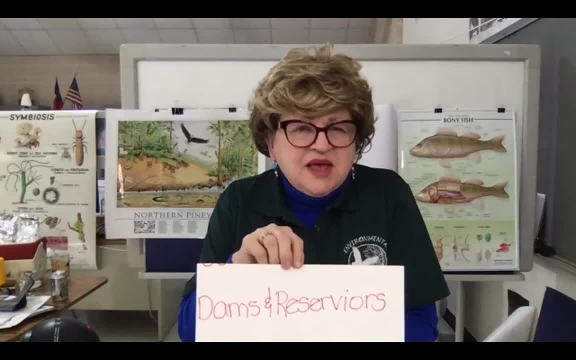 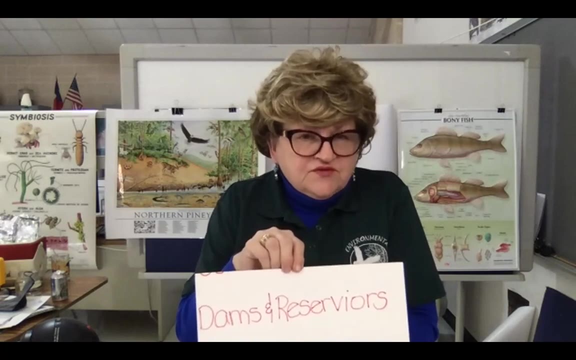 and the outside of the scale has the same kind of material that your tooth has. It has on it enamel. So the American Indians used to take these scales and make them into arrowheads to shoot arrows. So it's an interesting fish, It's a useful fish. They don't eat trout and crappie and largemouth bass and things like that. They primarily eat gizzard, shad and buffalo and carp. So they're not infringing on people who are into sport fishing. So anyway, the alligator gar is suffering. 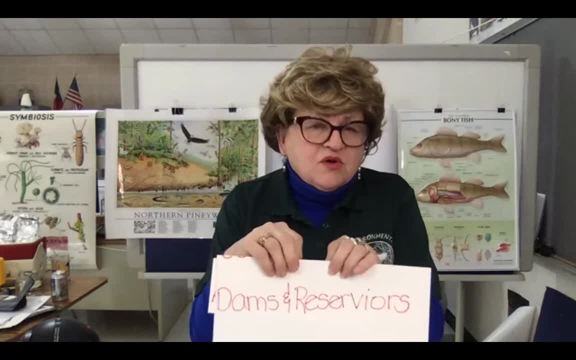 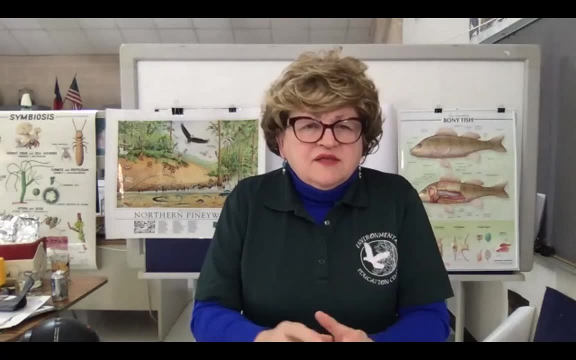 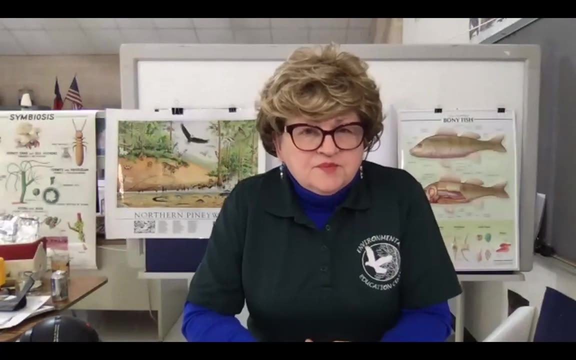 because of flood management or river management in Texas. So these are a couple of things to keep in mind. when you think about the things that people do to make things better, You have to think about all the different consequences. Mr Broughton would be glad to answer. 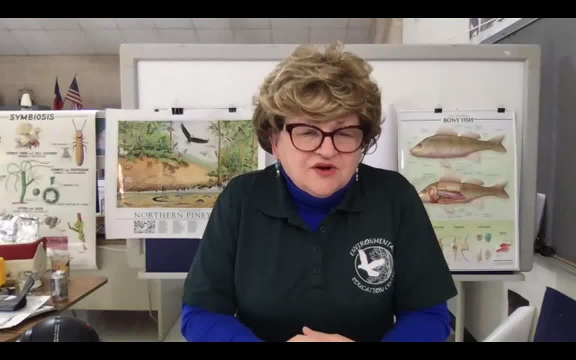 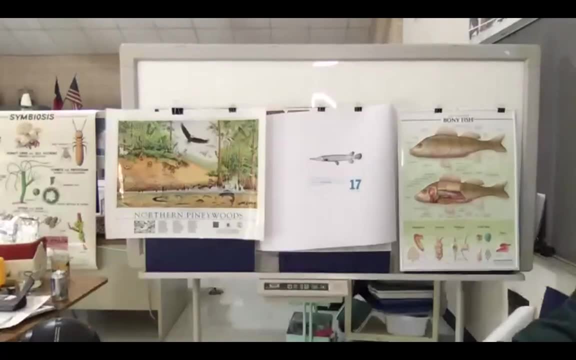 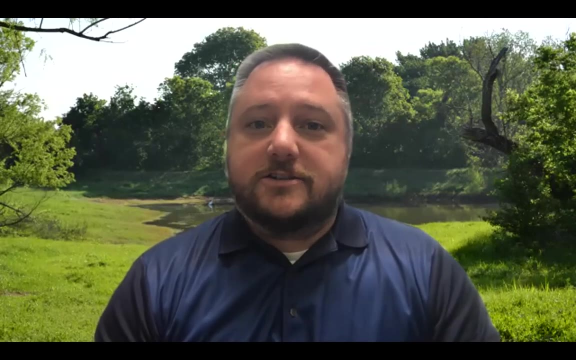 any questions you have about the lamprey or the alligator gar. Thank you. The question that came in was: are other animals suffering because of humans building dams and reservoirs? And I actually don't know the answer to that question, So I'm going to pass it on to Ms Nash. 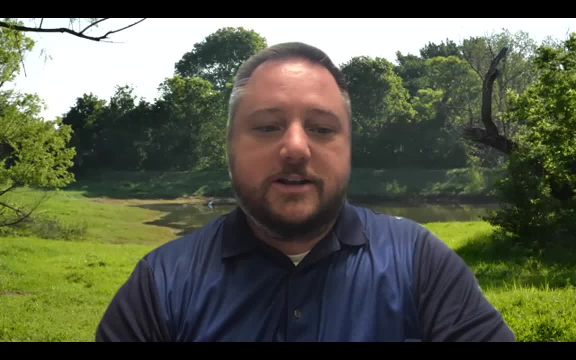 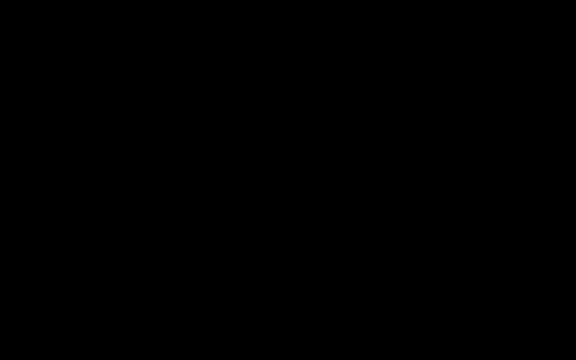 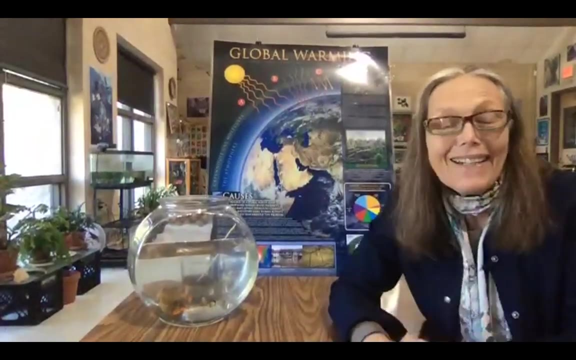 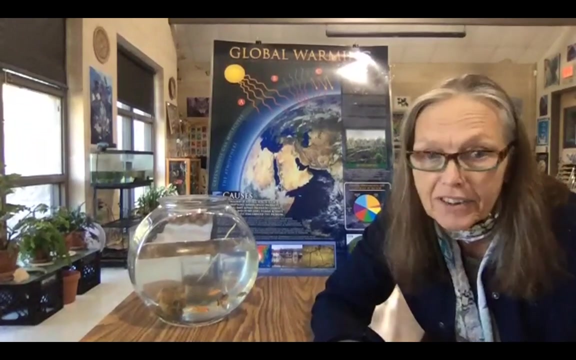 who's going to discuss how thermal changes affect aquatic ecosystems? And there we are. what a miracle. Okay, so welcome. welcome to my classroom students. And today, now we're going to talk about thermal changes. okay, Thermal meaning change in temperature. 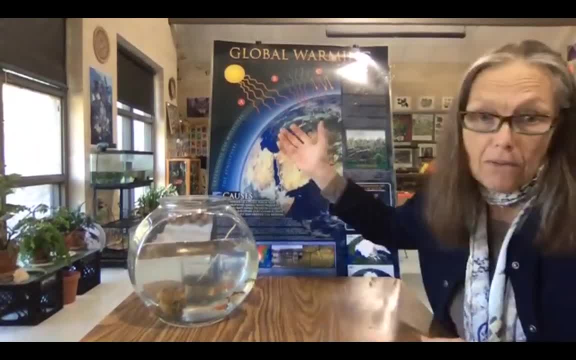 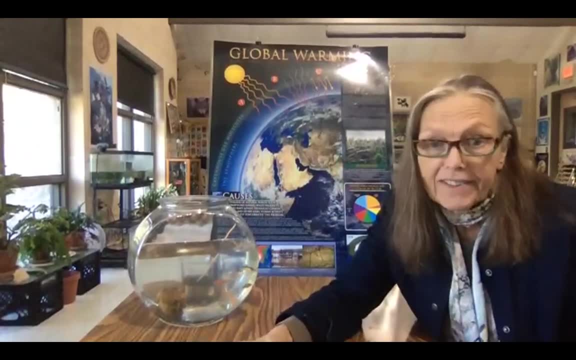 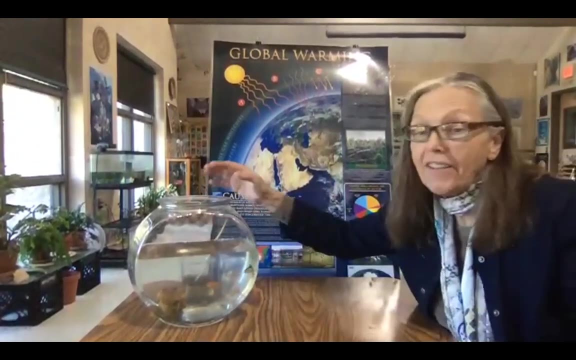 And so we've all heard, I'm sure, about global warming, And so global warming is increasing air temperature and water temperature, So water has been absorbing most of the extra heat that we have been producing And, as a result, a lot of bad things are happening. 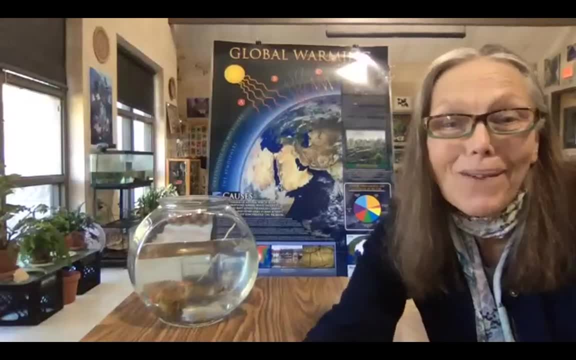 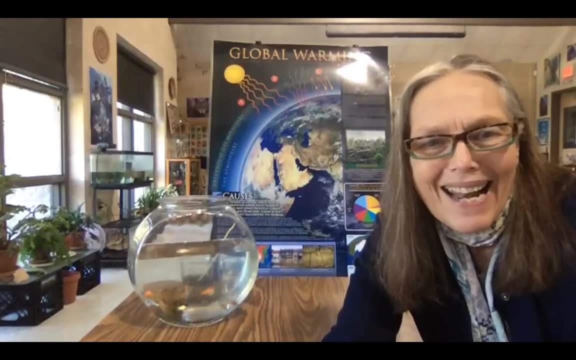 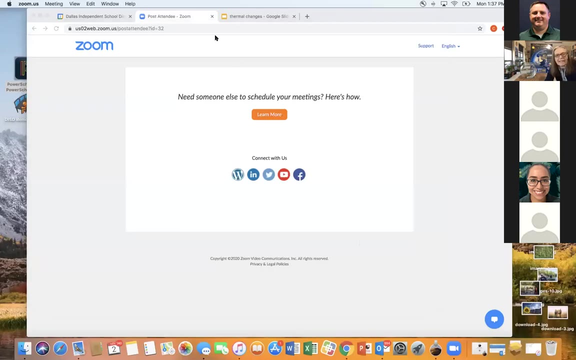 So we're going to review a few of them and then we'll think about what we could do. Okay, So I'm going to try to share my screen here, My screen, and share that one too, And then then, sorry, go over there. 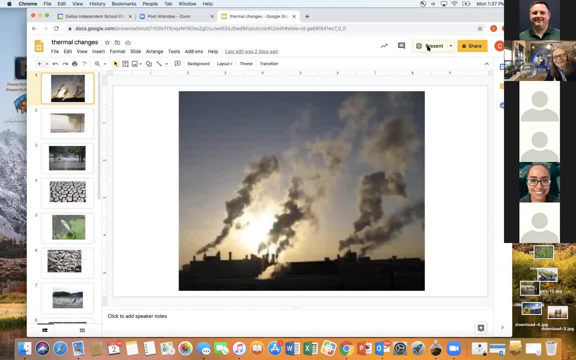 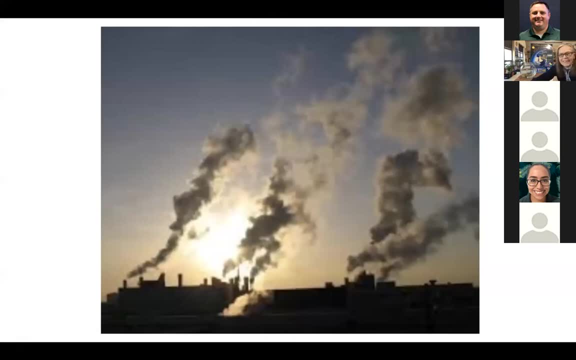 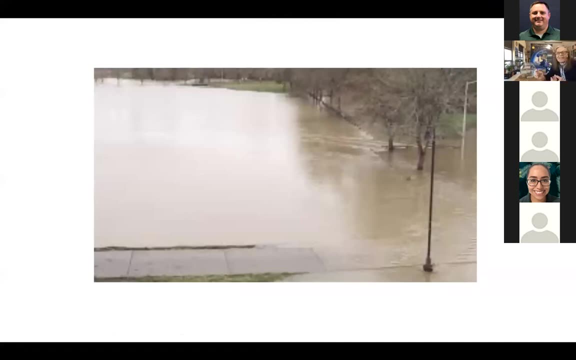 Okay, So here we are, And so, as we mentioned before of industry, co2 in the atmosphere leads to two things: um, basically extreme weather events. so we have lots of flooding events in houston, just increases, runoff, all kinds of things to go in, but this is because of that: extreme weather events, okay. 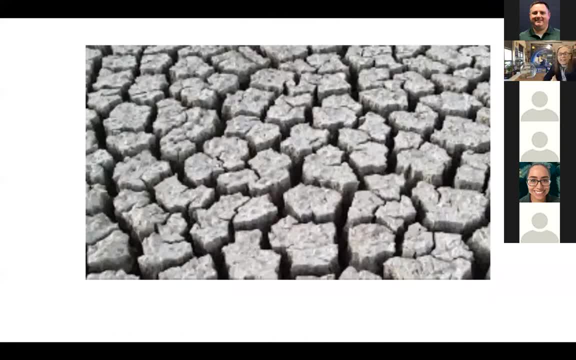 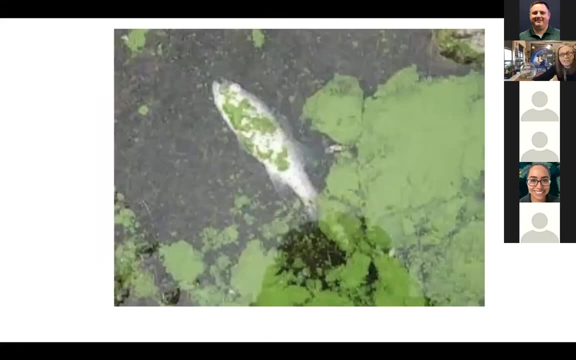 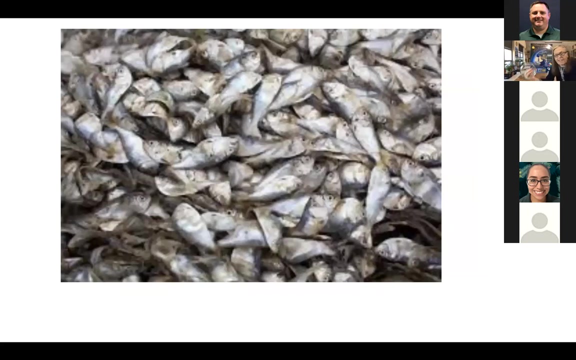 it also increases drought. so not only drought, but not only floods, but drought- they kind of go together really oddly enough. so our, our own little ponds have dried up completely okay, and of course that leads to dead fish, um, lots of dead fish as the water gets hotter. some species can't take it okay because the water gets hotter, you hold less interest, so oxygen, and then the fish die. fish in other organisms die, Some fish quickly invasive, like these amazing Asian carp and our own carp that we have around here, the common. ones are able to survive warmer weather. So the species change as the temperature changes. some can take it and some can't, And in particular, the invaders tend to be able to take it. Invasive plants, so elephant ears- okay, they were brought in as an ornamental. 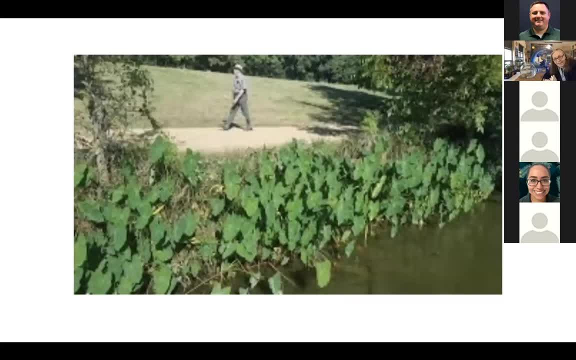 you have seen these in people's gardens. they are not native, they are tropical and they should be dying in the winter. but as things get warmer, as winters are warmer, that's cold time- These kinds of plants- this is an aquatic plant, semi-aquatic aged plant. 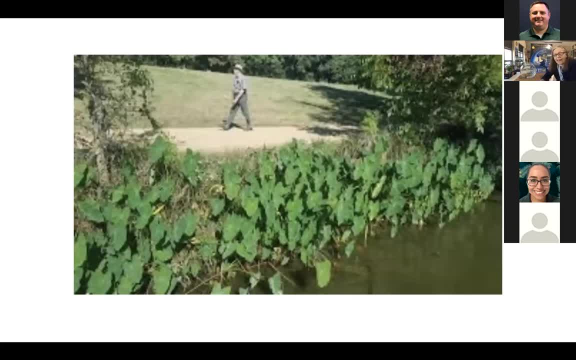 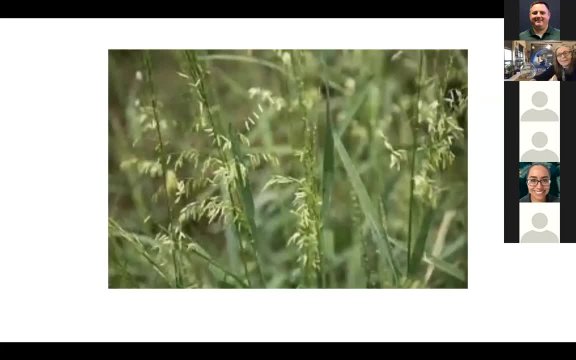 crowd out the native species, And this is a particularly sad one. this plant is Texas wild rice, And who knew that Texas had its own very, very rare species of wild rice, Like we all know them up in Minnesota and Canada they have wild rice, But this is our. 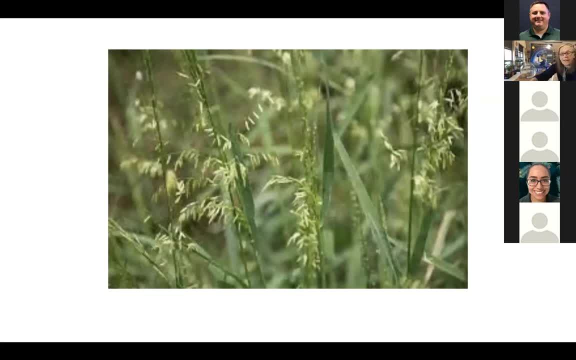 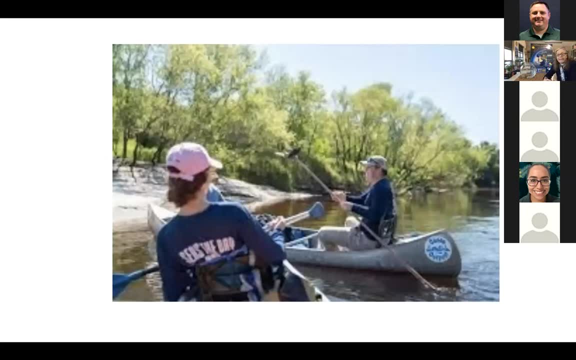 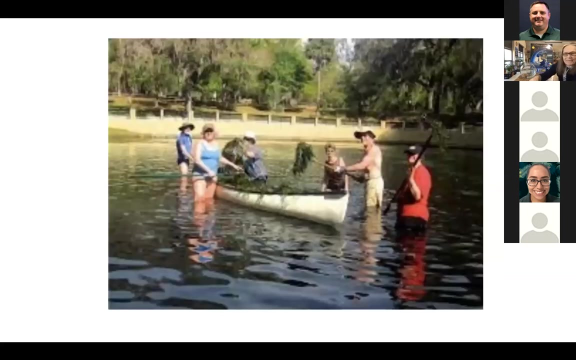 own, very rare, being crowded out by those elephant ears. So what can we do? What can we do? Well, these people you may not be able to see have speared a- hopefully yummy- invader, So we can eat them. We can eat the invaders in the case of fish, Or we can just 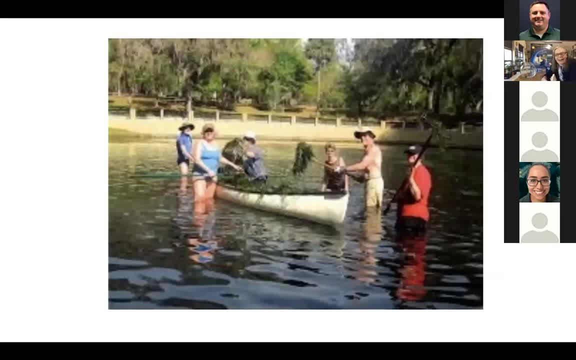 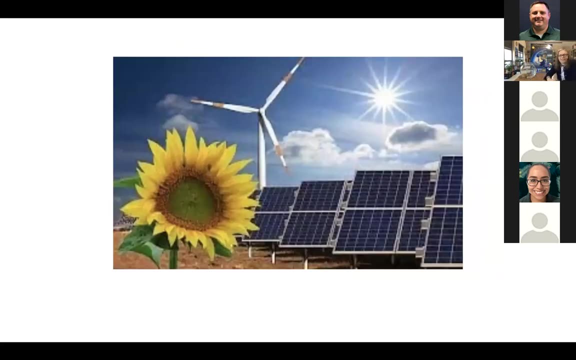 pull them out in the case of plants. So these people are pulling out some invasive hydrilla, I think, from a lake down in the hill country. So we can get involved And do what we can- Other things we can do to lessen the amount of heat that's affecting. 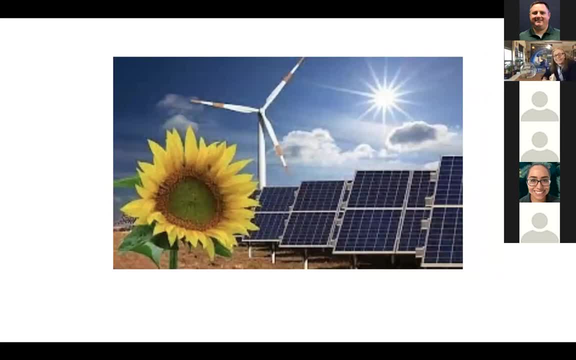 our atmosphere, our oceans, our rivers, our lakes is to use alternative energy Like solar energy, wind energy, geothermal energy. We can use biomass from plants we can grow. eat less meat. All these things can help reduce levels of CO2, drive less. use your breath. 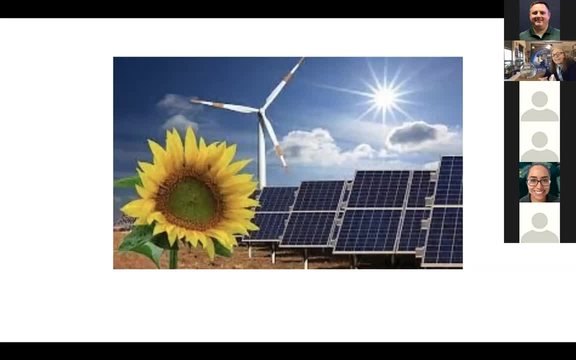 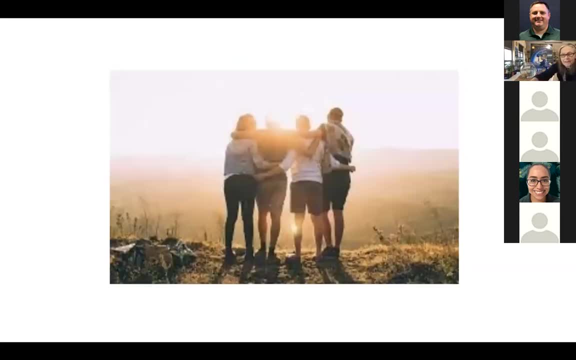 before you drive your bike instead. All these things can reduce the levels of CO2, and therefore reduce the heat in the atmosphere and in the water. We have to work together to do this, All of us together. We have to educate ourselves, Work together And we can try to make our 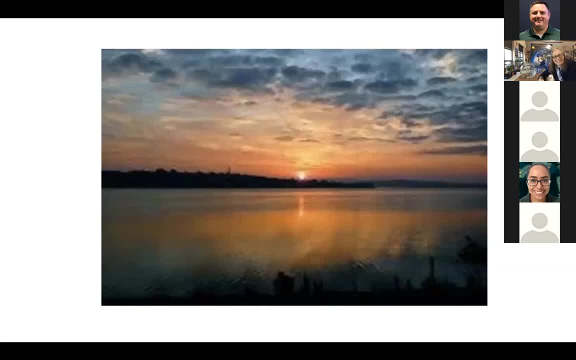 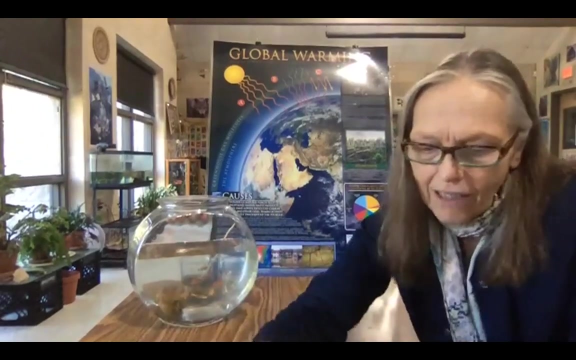 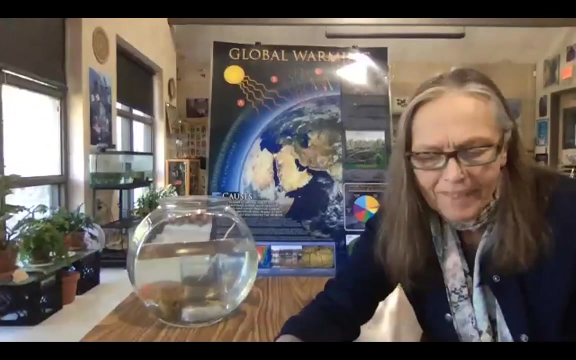 beautiful lakes and rivers and oceans, a habitat for all the animals and animals And plants that live there. There we go, And now I'm going to stop sharing. Stop sharing, And okay, I'm going to stop sharing. Okay, I'm back, I'm back. actually, I hope I'm back. Okay, Done So. thermal changes. 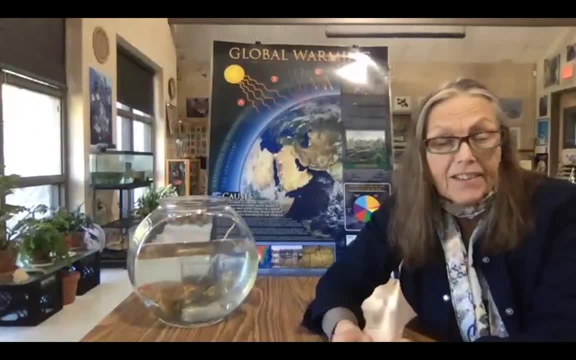 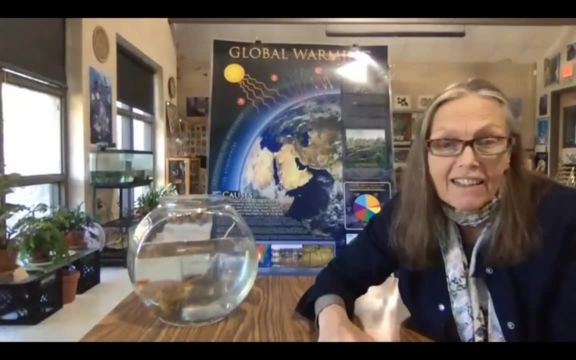 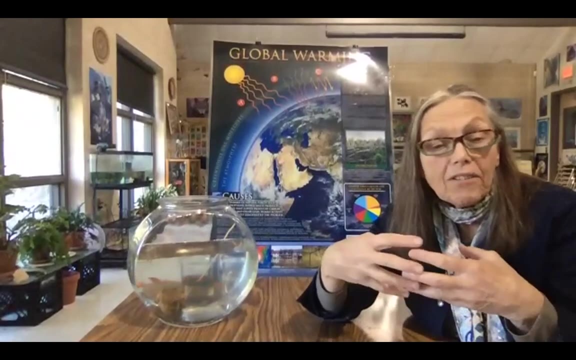 are happening all over the world, But water in particular, because it absorbs heat. it's absorbing more heat than the land in particular, And it also has a lot of what we call thermal inertia, And so, in other words, it takes a lot of energy to change the temperature of the water And once it's, 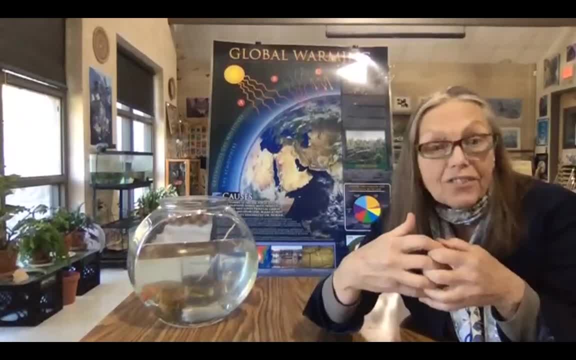 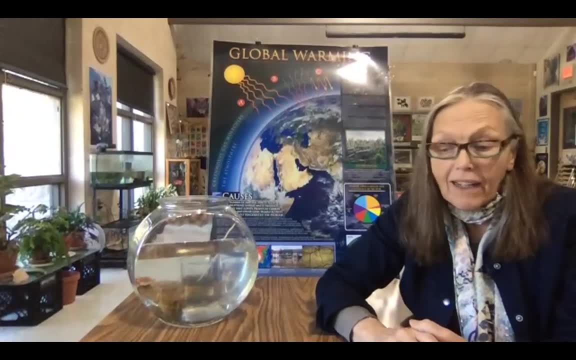 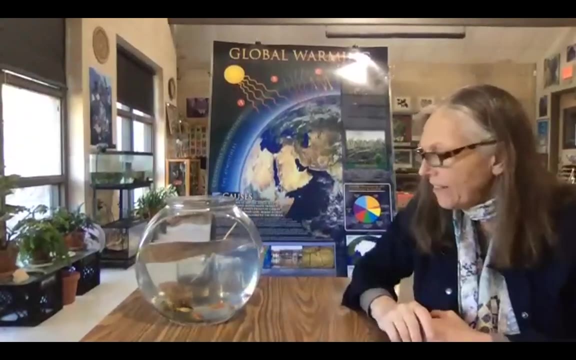 a certain temperature. it takes a lot more energy to change it back. So we need to be aware, Aware of what's happening around us And do what we can to help our little fishy friends. All of these are not wild fish, It's all goldfish friends And that's all I have. And 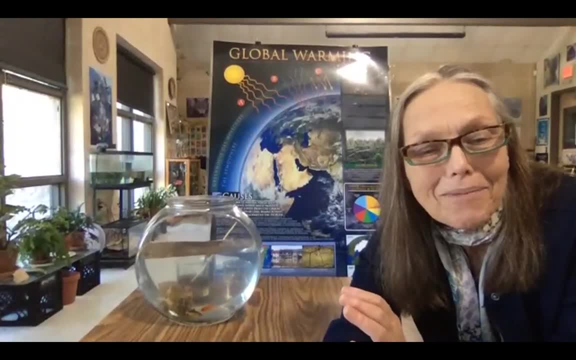 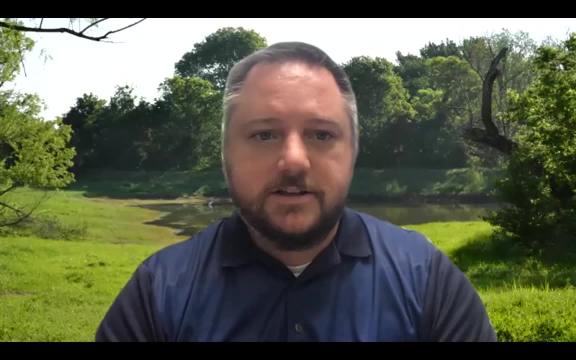 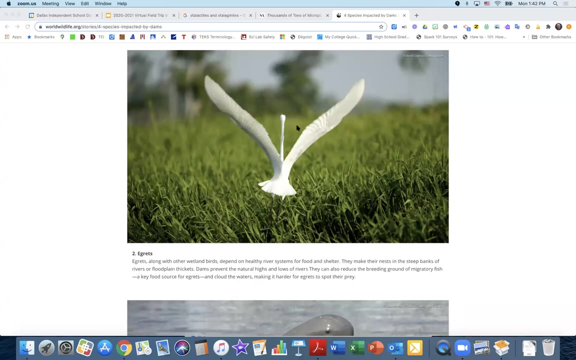 if you have any questions, you can ask Mr Brodden. Thank you, Ms Nash. I'm going to share my screen here so that I can show a couple of things, And the first one is: I found the answer. So if you're using an ultrasound, you can see that it's showing the temperature drops. 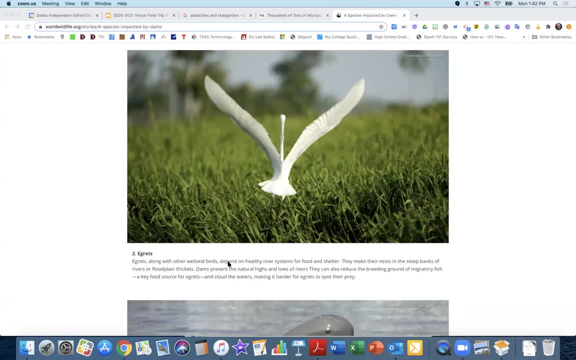 down toward about 20 degrees from where it's supposed to be right now, And it looks like it's up to the authorities to tell you about that. It looks like we're in a little bit of a mud hole here. The controls are going to have to be aligned with the meters.